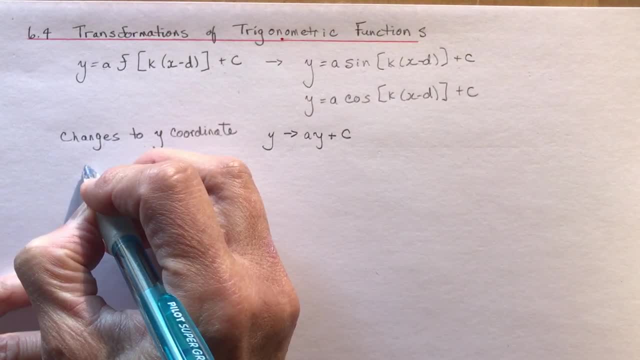 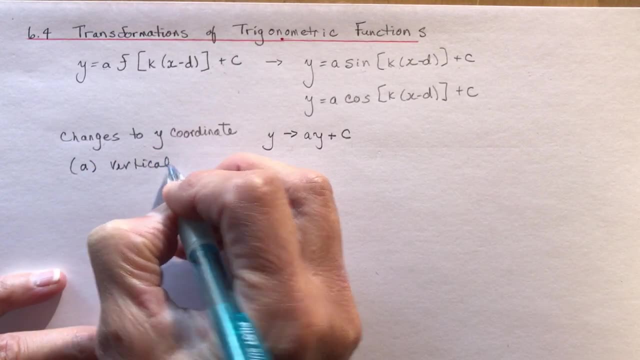 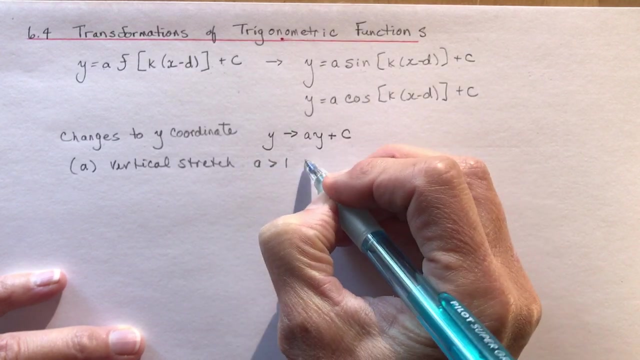 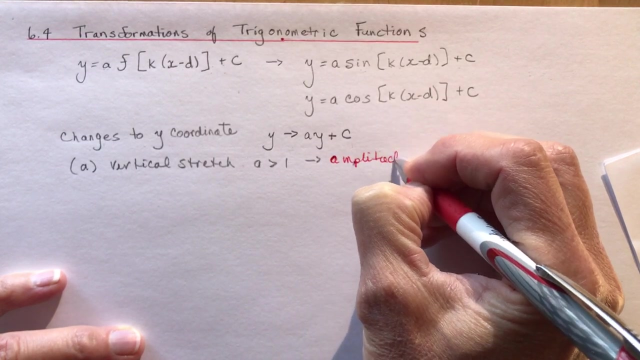 Now do you remember what the a does? Of course you do. A means Vertical stretch or compression, right? So it's a vertical stretch if a is greater than one. So, if a is greater than one, and this is affecting, let's write these in color. So you've got this. this is an amplitude for my graph, right? The a value is amplitude in this for trig functions. 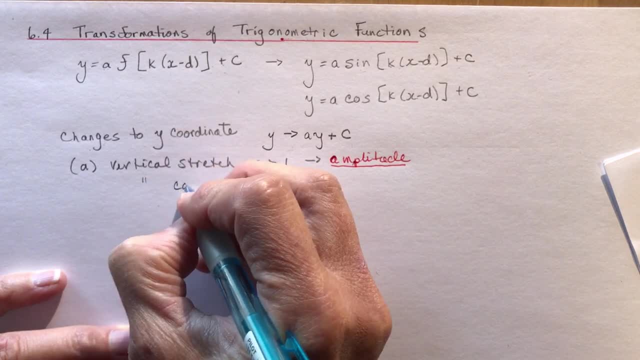 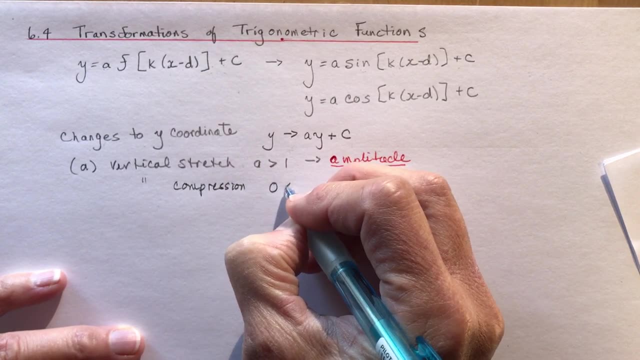 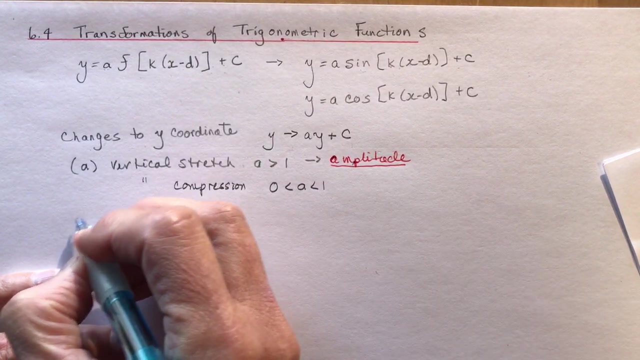 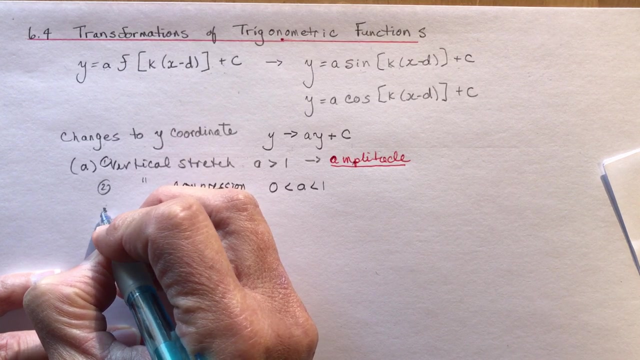 So if you have, you have a vertical compression and you know what that looks like. That means we're going to make a between zero and one. Everyone else said: well, what about the negative? The negative means a reflection, right, So that comes in another section here. So we have a stretch, or it could be compression, or, third, we can have a negative. 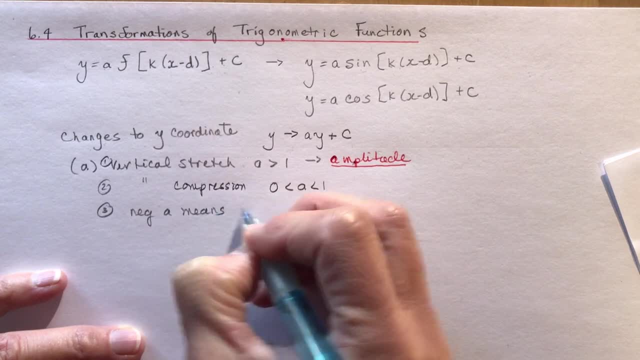 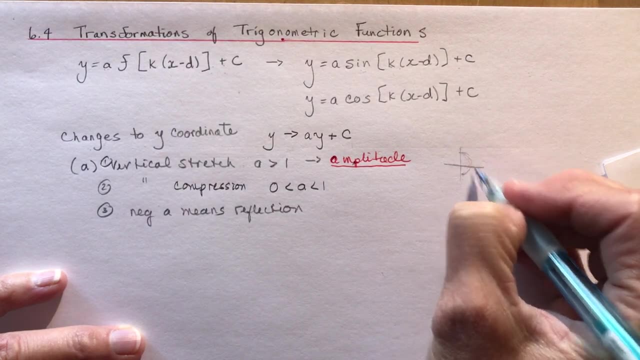 Negative. a means reflection about And remember, if you have trouble remembering which one you're affecting: y's. So the y's are going up, The y's are going up and down this way. So it's reflection about the x axis. 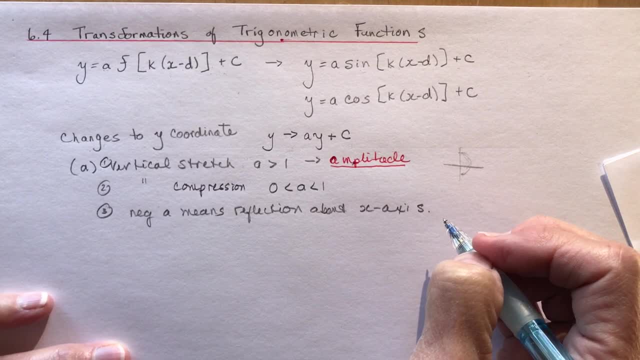 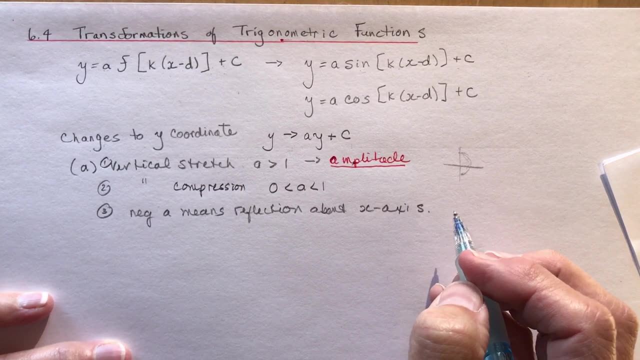 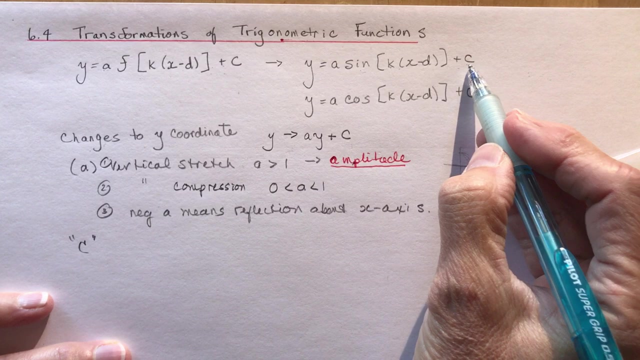 Okay, so we have negative and positive, sine and cosine functions, and we're going to take a quick look at that in a minute as well. Okay, so what does the c do? So c is your vertical shift up or down. c units. 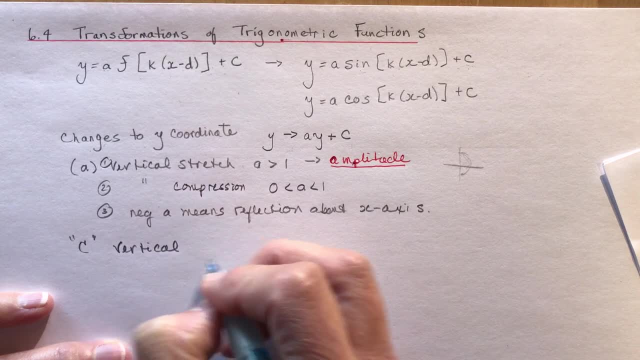 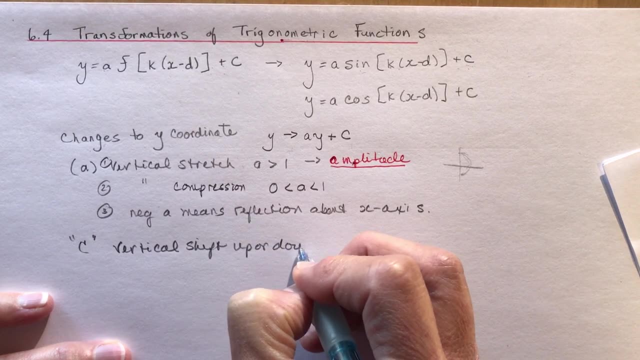 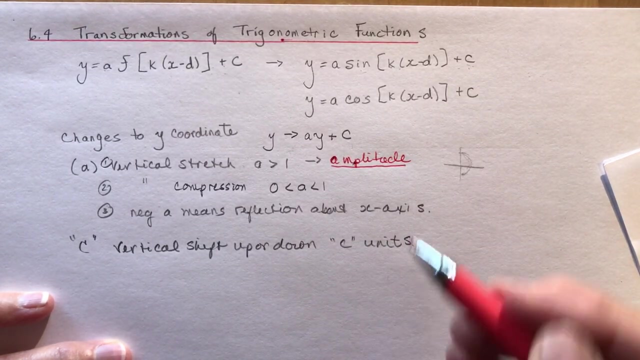 So, in terms of our functions, our trigonometric functions, trigonometric functions- let me just write this down so I don't make a mistake- vertical shift up or down c units, c units and that's affecting all together. now one, two, three, that's the axis. 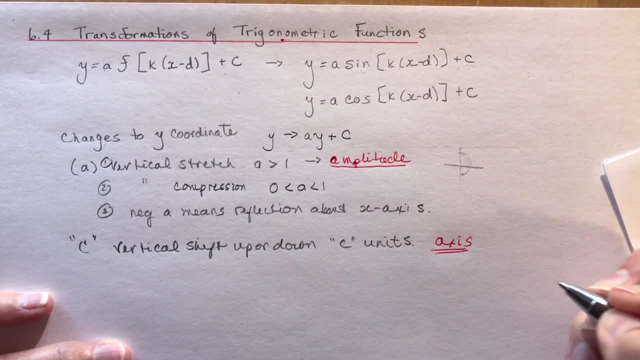 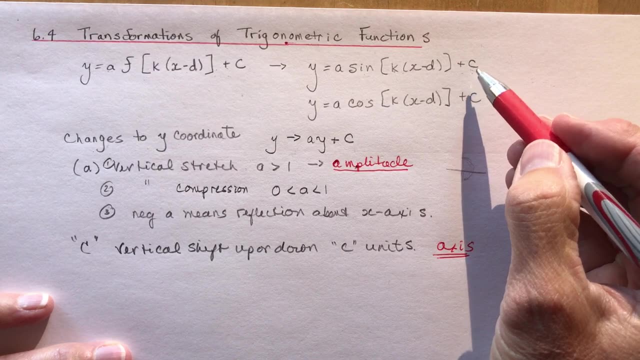 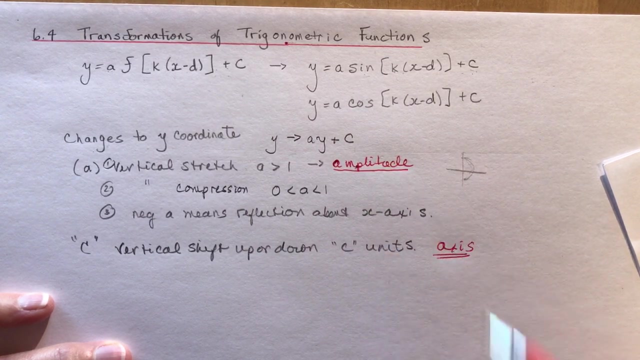 it tells you where the axis is going to be. so if I have plus five here at the end, your axis is going to be at five and then you're going to adjust your amplitude from that axis. so amplitude for the a value and the axis, amplitude and axis, those are the two important changes to the y coordinate. so 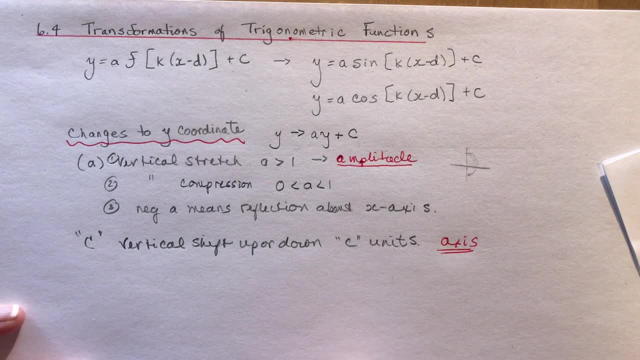 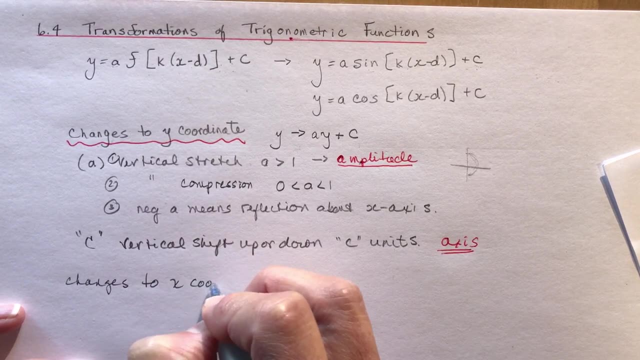 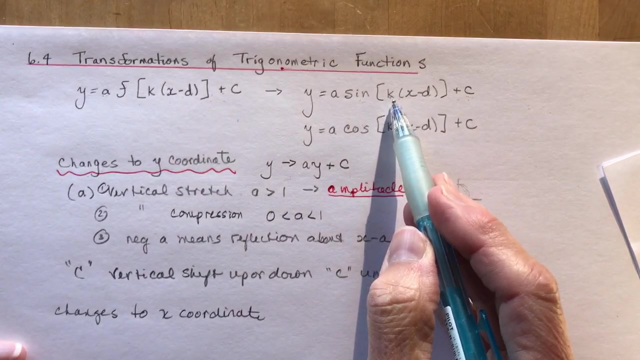 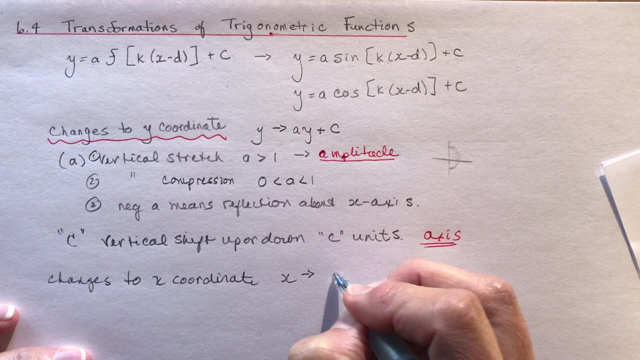 let's take a look now at the x, because everything's a little bit different in in trig than it is in other transformations: changes to the x coordinate. so if I was going to ask for a mapping rule for my x, you'd say I have to do X divided by K, divided by K C plus D. so X goes to X. 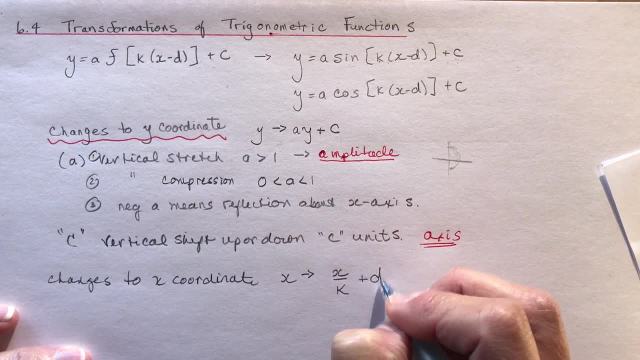 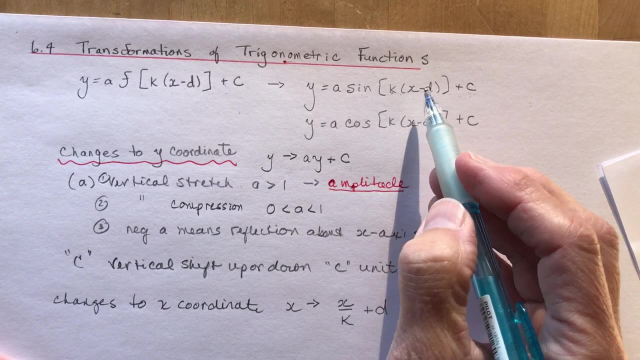 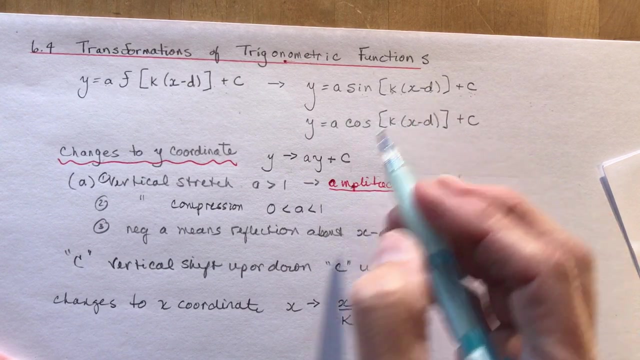 over K plus D. so, like I said in the grade 11 course, X's are weird. it's all backwards, it looks like times a K minus a D, but you're going to divide by the K and add D or change the sign here. okay, so the K is important because it. 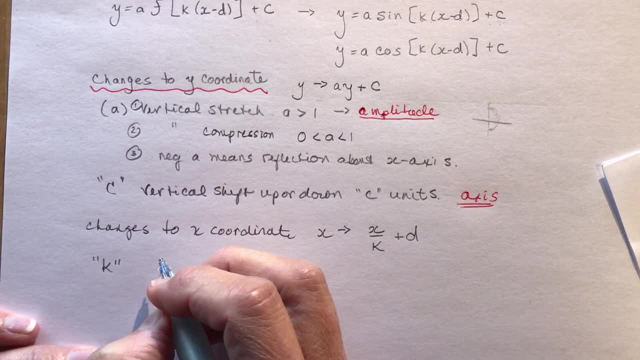 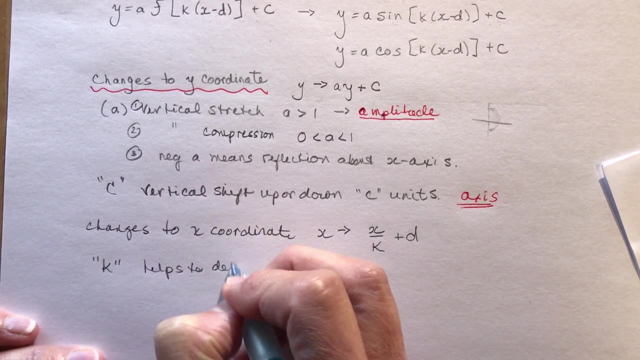 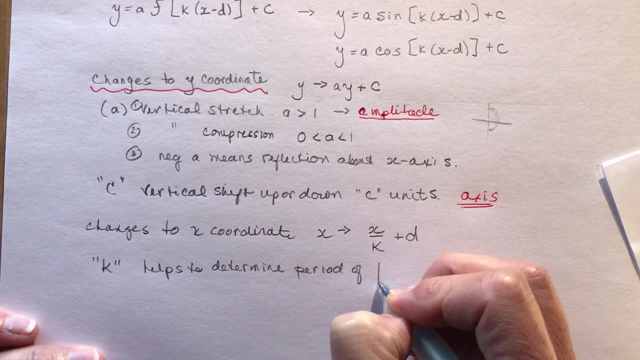 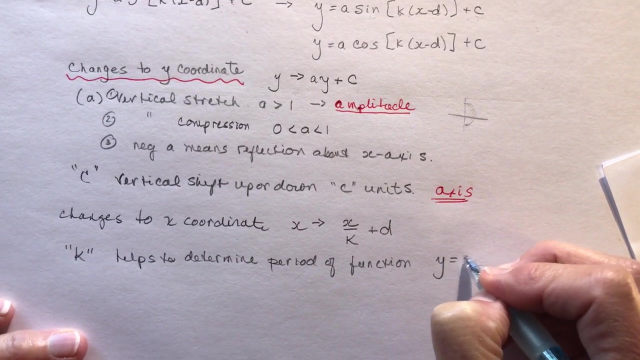 determines the, the period of your trigonometric function. so K helps to determine, to determine the period period of function, and this is a little calculation that you will need to do over and over again because, if you remember, Y equals sine theta or cos theta has a period of. 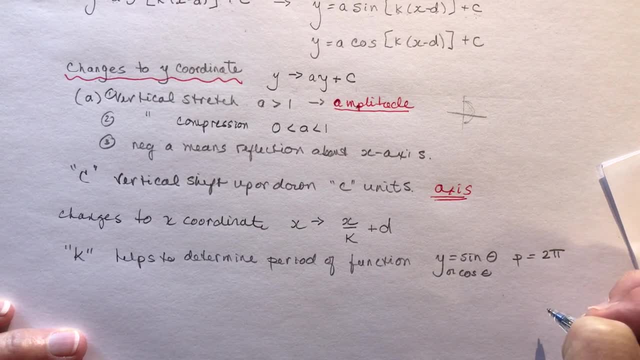 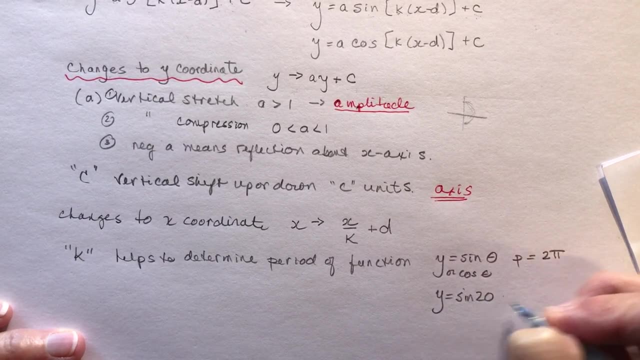 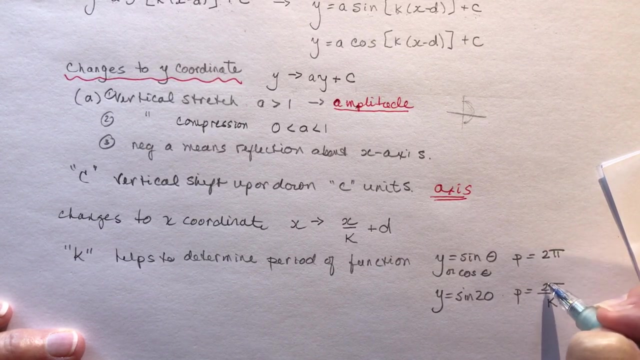 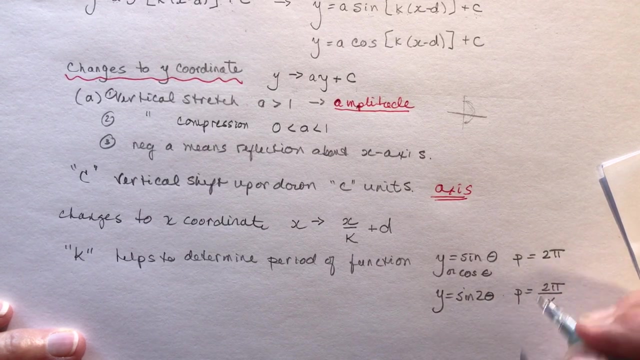 2pi. so if I want to know what the period is of Y equals sine 2 theta, the period is 2 pi over K. okay, so you have to always divide the period by the K value. so in this case the K is, k would be 2, whoops, I should put a little sign there. so the period would be pi. right, so 2 pi. 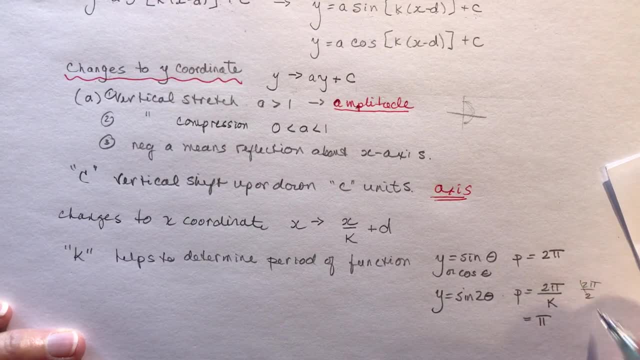 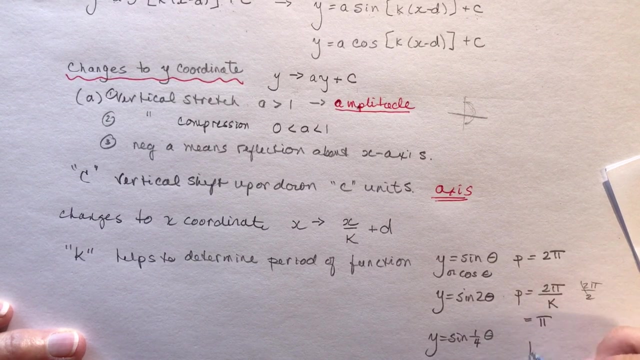 divided by 2, 2 pi over 2 pi. Okay, so um. alternatively, if you had the period- let's say I had um y equals sine 1 quarter theta- then the period would be 2 pi over 1 quarter. so remember. 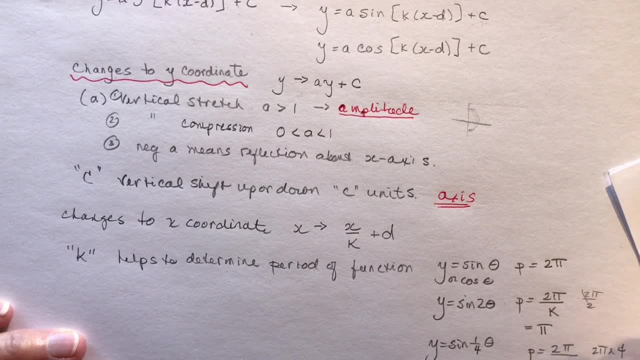 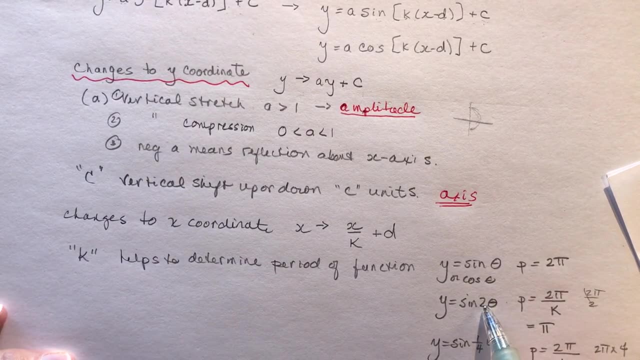 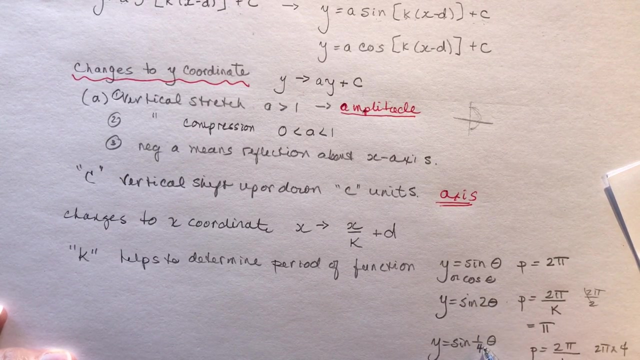 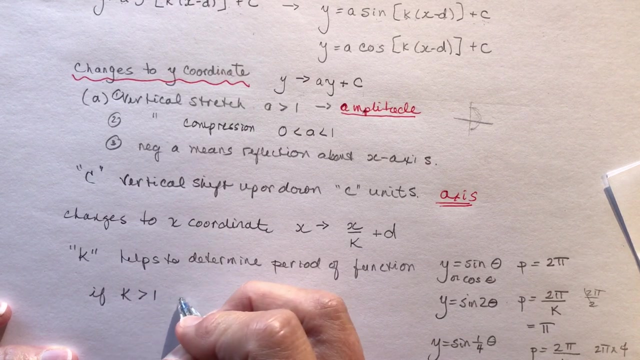 that's 2 pi times 4,, which would be 8 pi. So recall now that a 2 here- or a number greater than 1, results in a compression and the fraction gives you the stretch right. so if k, if k is greater than 1, then you have a horizontal. 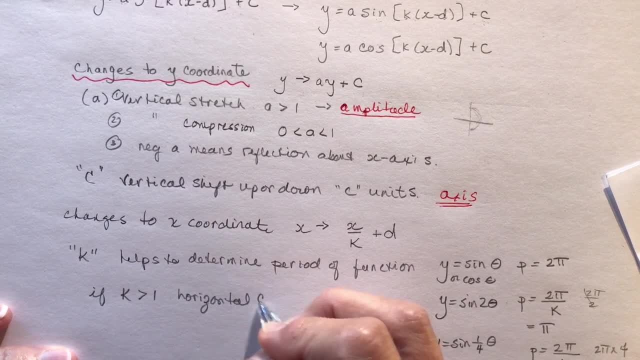 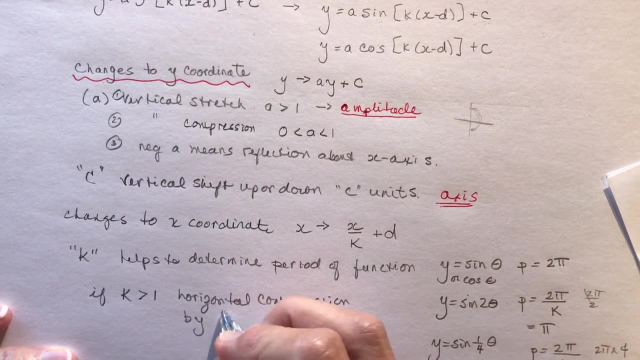 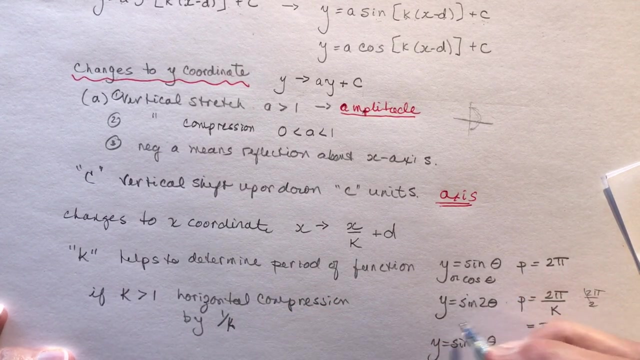 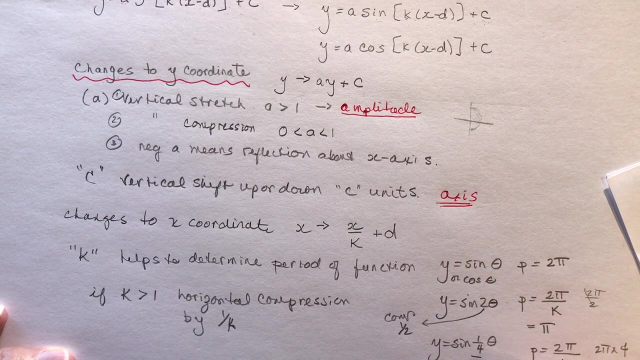 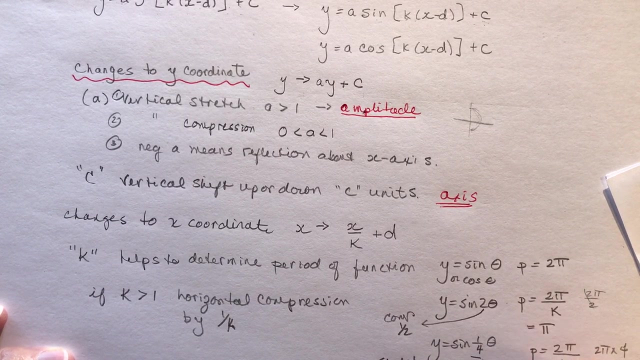 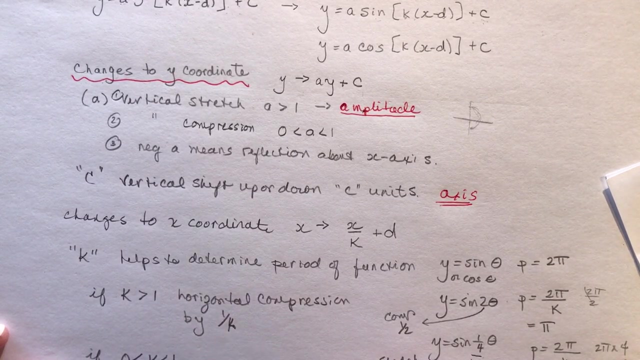 compression by 1 over k. So in this case here we had a compression of one half right, so this one would be compression of 1 half and this one would be a stretch times 4 right, 1 over this. so if K is between 0 and 1, in other words a fraction, then 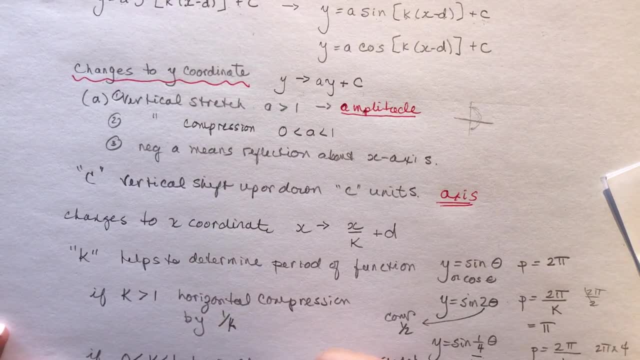 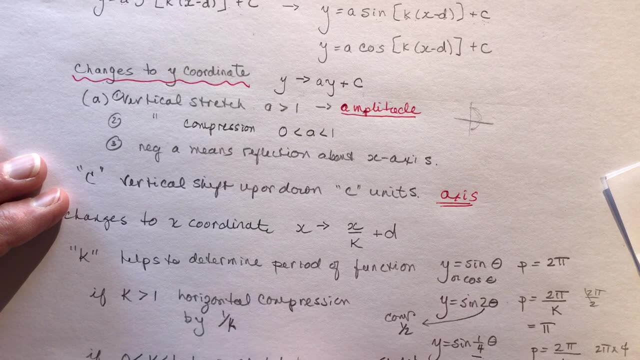 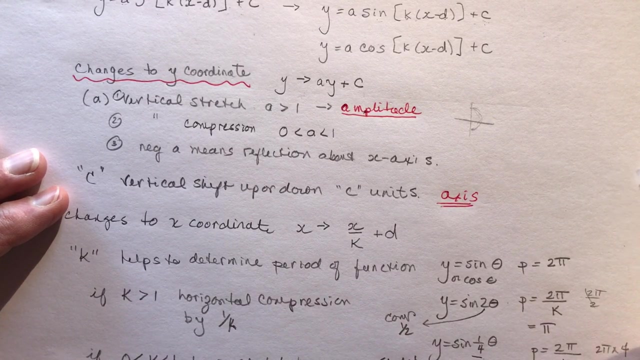 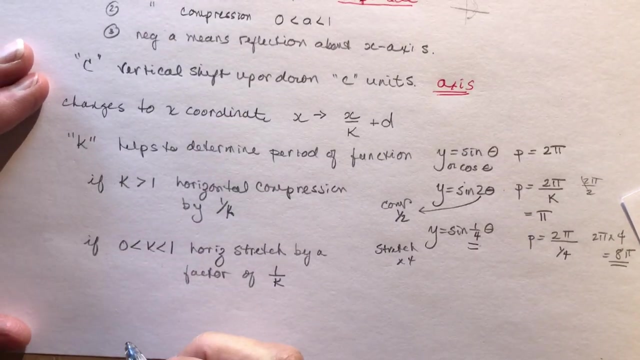 it's a horizontal stretch and that's changing again. it's changing the period of the function horizontal stretch by a factor of 1 over K again. so you have to remember how to divide your fractions, right, okay. so what else do we have left to do here? we need D, right. so we have. D tells you. this is the horizontal shift. 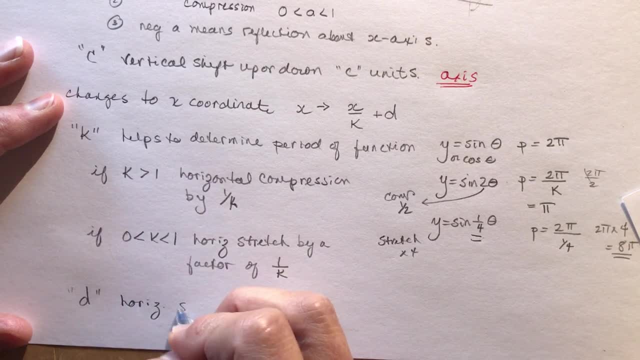 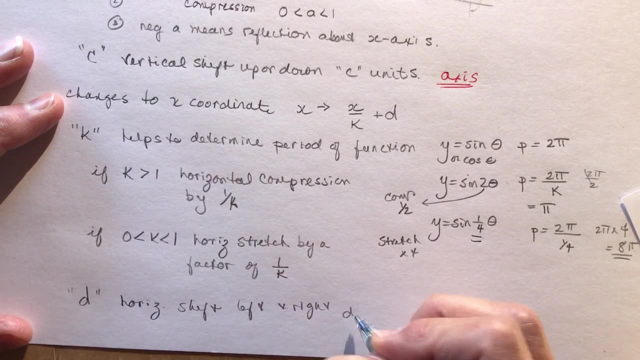 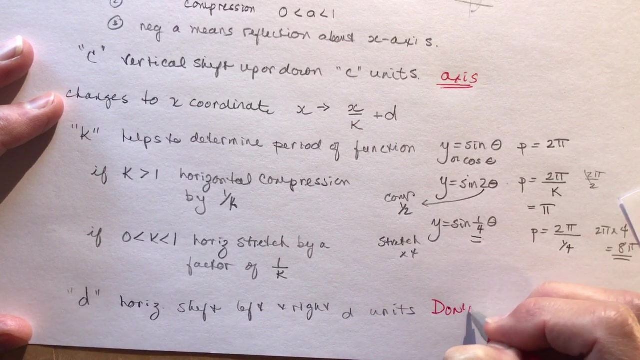 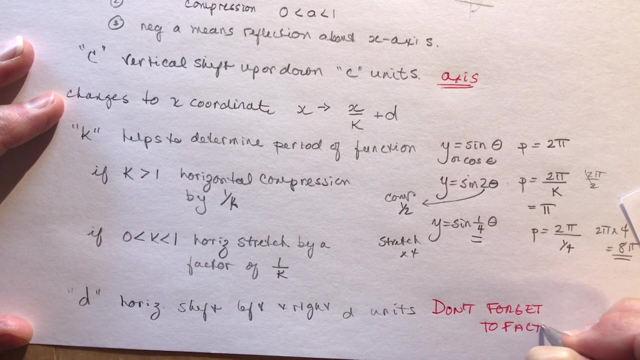 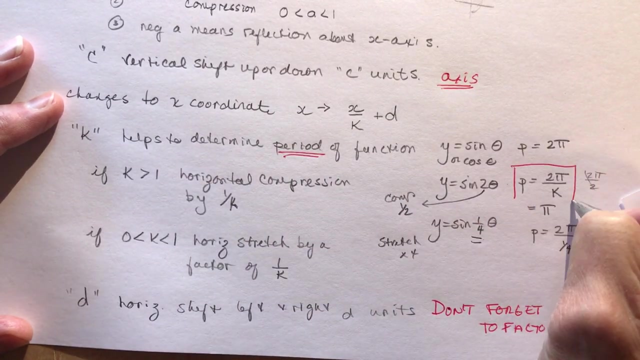 left and right, horizontal shift left and write d units. and I can get up my red pen right now and write: don't forget to factor. I'll do an example in a minute. don't forget to factor. okay, so the k helps determine the period. and this little formula here- period is two pi over k- is very important, vip. okay, that formula. 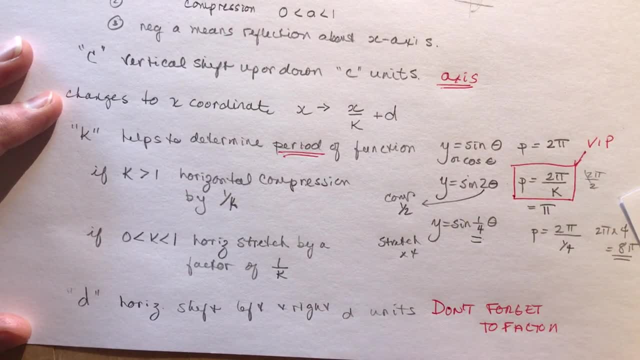 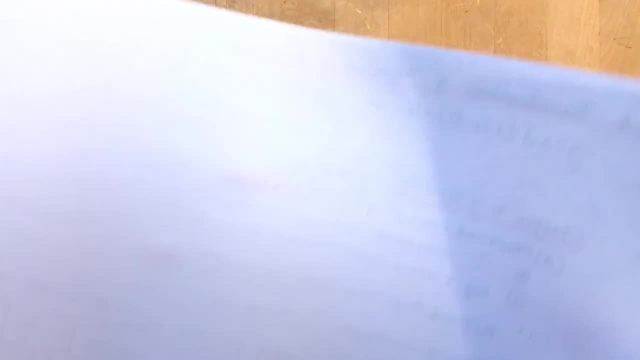 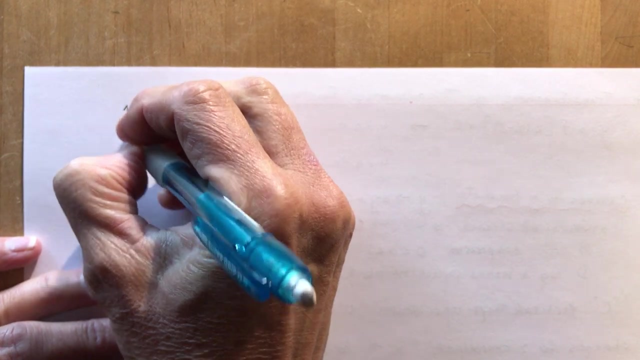 you're going to use that lots to find the period of the function. okay, let's do an example, flip this over. and we're going to do: um, let's make up a good one for you, get pencil going. so we're going to say y is equal to. 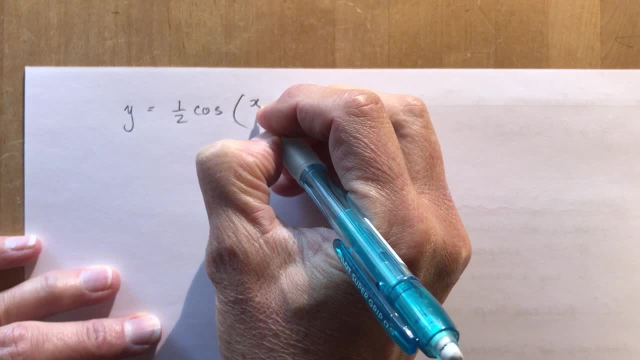 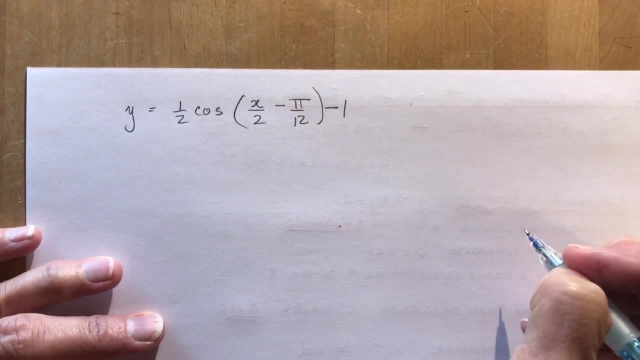 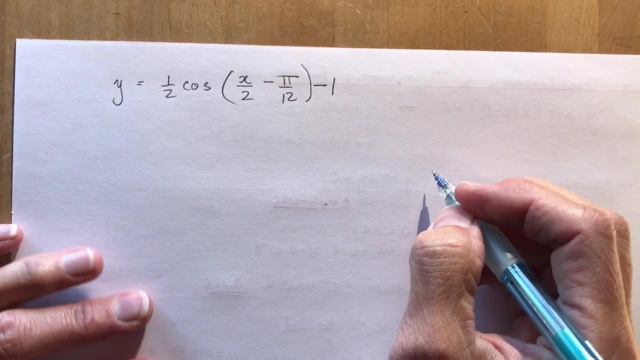 one half cosine x over two minus pi over twelve minus one. your job is to graph this function, state the transformations. we can state them as we're doing them. let's figure out what the mapping rule would be first. we could do some key points. you've done that before, so you can either use: 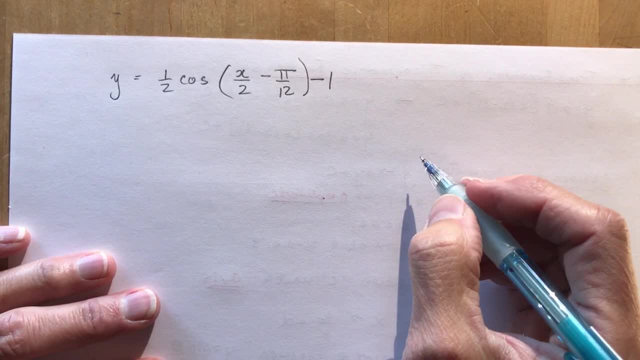 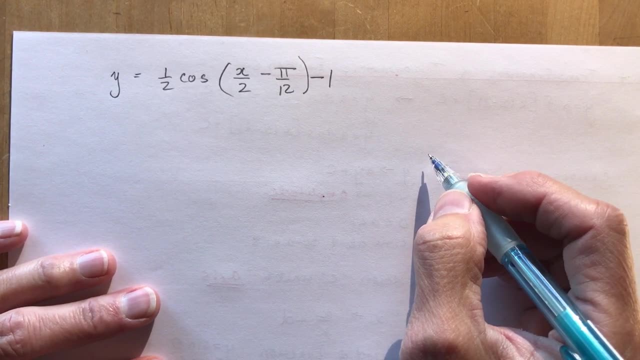 key points, or sometimes you can just eyeball these functions. so it's two kind of different methods, but But one you might feel more comfortable with than the other, But I'll show you both. Okay, so I have 1 half cos x over 2 minus pi over 12.. 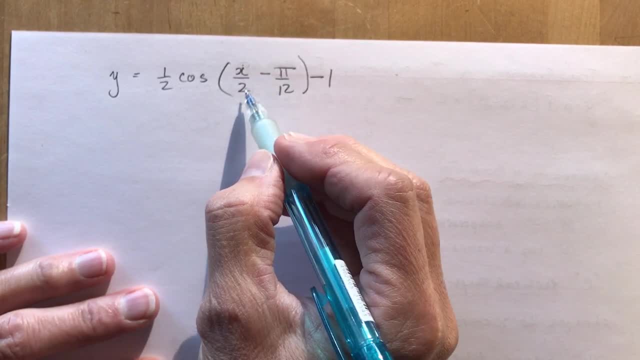 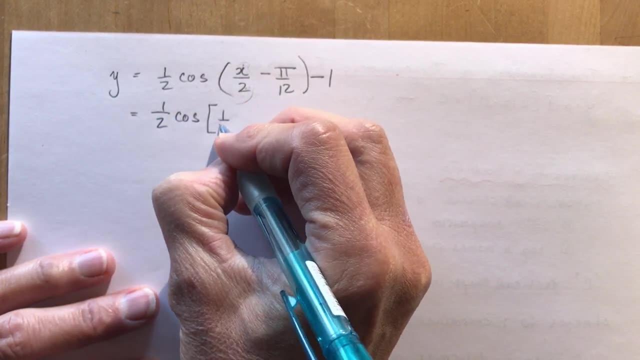 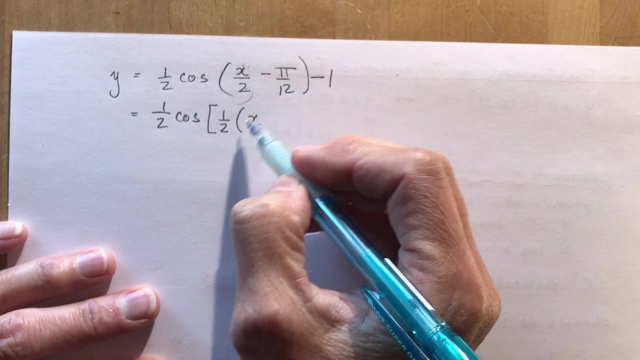 So right away I see that I need to factor this: This isn't x, it's x over 2.. So I rewrite it: 1 half cos big bracket. Take out a half. That leaves me with x. And please be careful when you divide minus pi over 12 by a half. 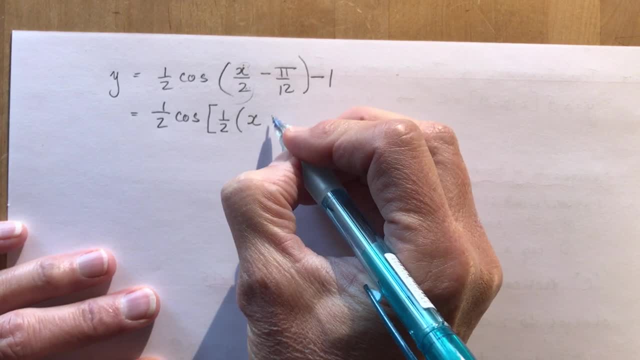 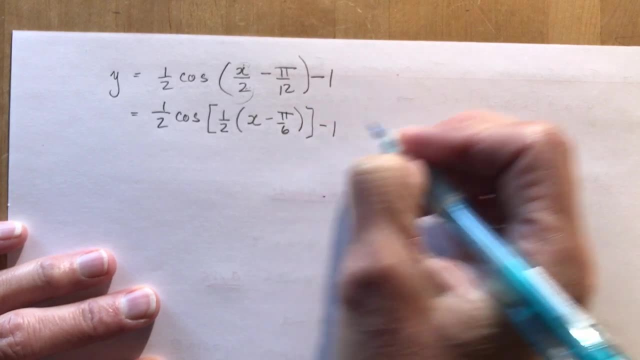 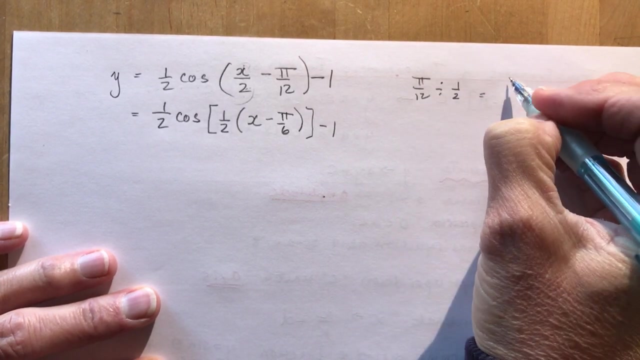 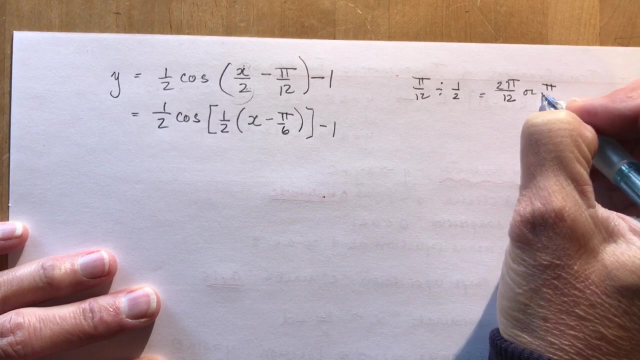 What should your answer be? Please don't say pi over 24.. It's going to be minus pi over 6, minus 1.. Okay, because pi over 12 divided by 1 half is 2, pi over 12 or pi over 6.. 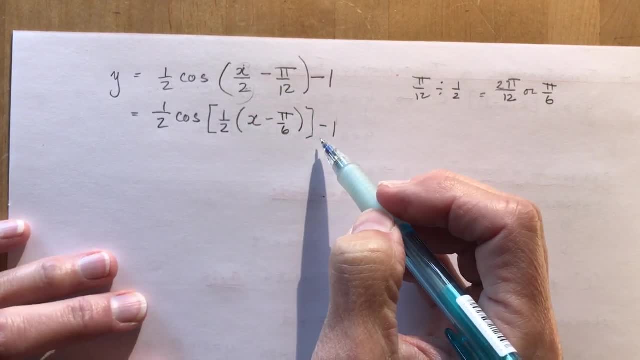 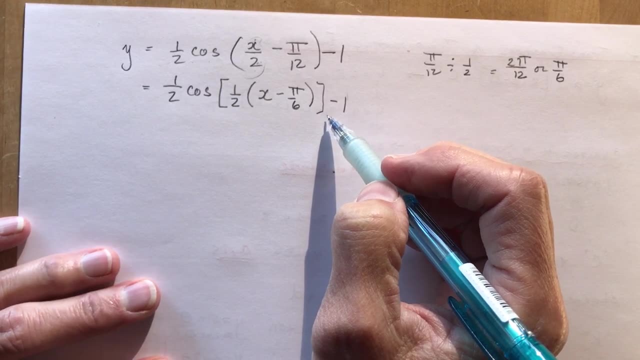 Okay, so be careful when you're dividing fractions, Don't make that mistake. It's kind of very sad. It's sad to be doing that in grade 12 for everybody, including your teacher, who won't want to even mark it. Okay, so here's my mapping- not my mapping rule, but my transformation. 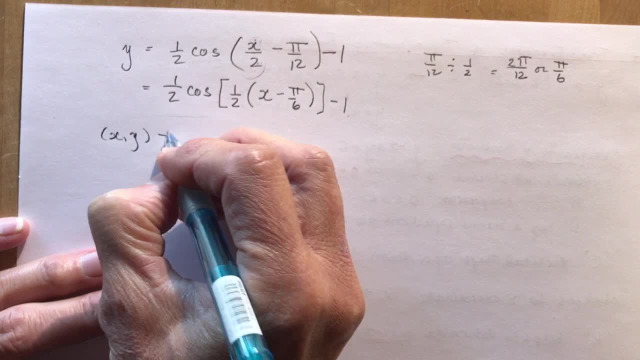 And I'm going to state the mapping rule now. So I'm going to say: I take my x's and y's And what do I do to my x's? Well, let's do what you do the y's first. That's always easier one. 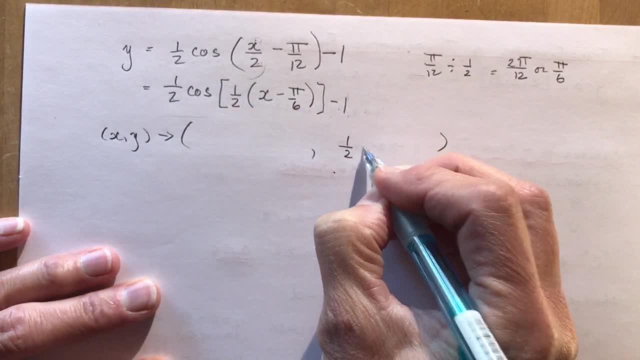 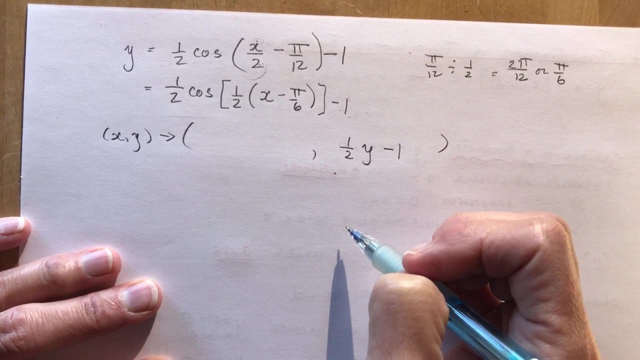 1 half y minus 1.. 1 half y minus 1.. Very easy Why you should never make a mistake with- And now they should You make a mistake with x, because we have 1 half, So we're dividing by half. 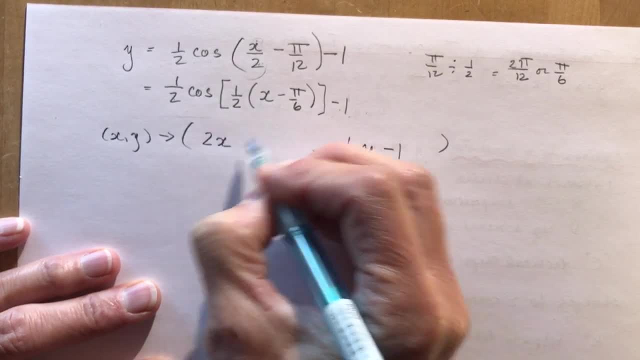 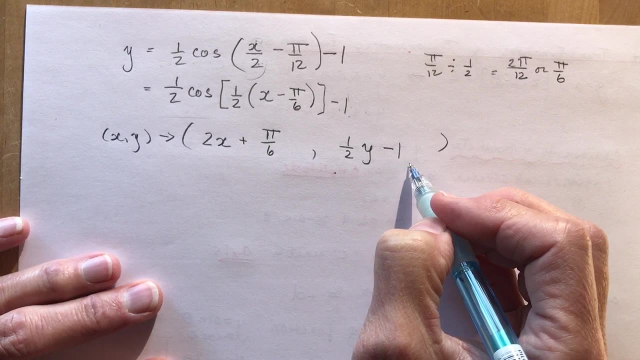 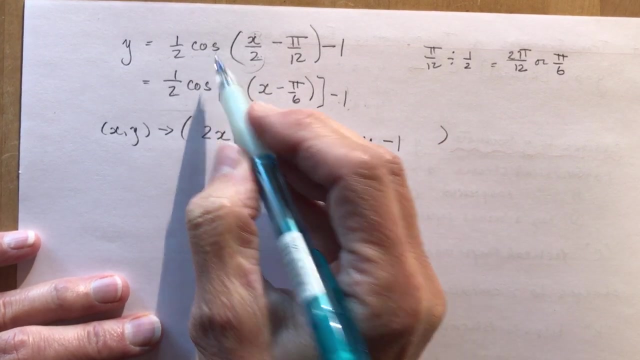 That means multiplying by 2.. So I have 2 x's and not minus pi over 6, but plus pi over 6. And there's a beautiful little mapping rule for you to use with some key points of the graph. So I'm transforming a cosine function. 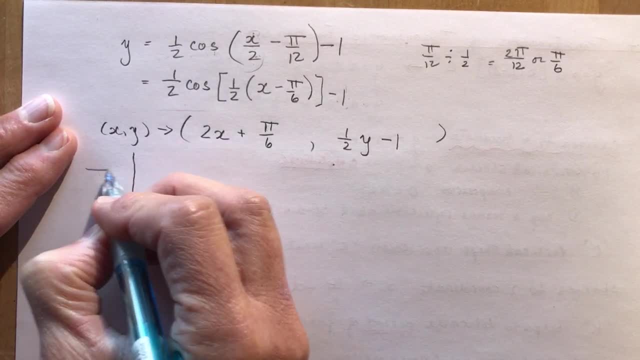 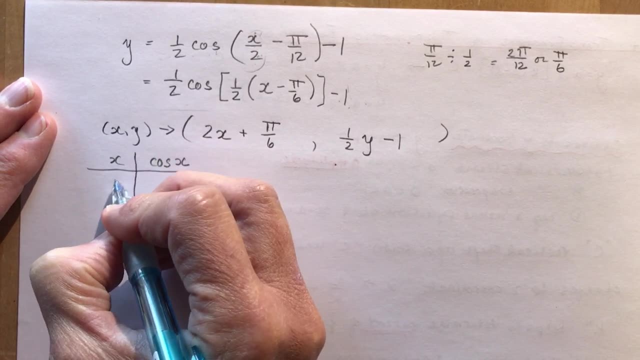 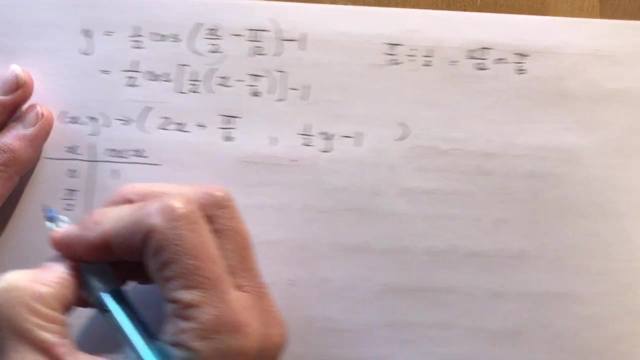 So it would probably be a good idea to have some points for the cos function. So I'm going to do x and cos x. So if I did 0 and 1.. So I'm using just the basic cosine function here that you should be able to draw very quickly. 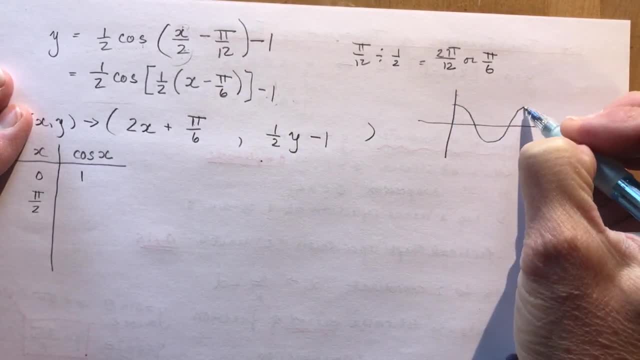 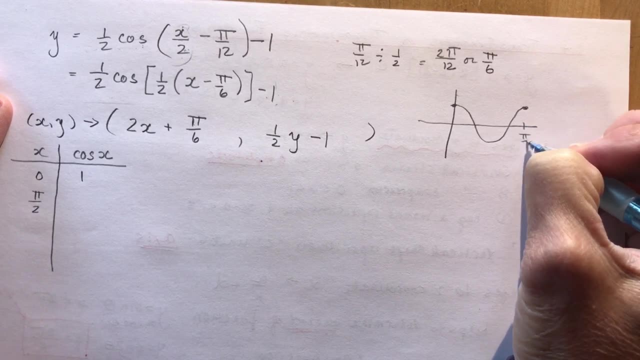 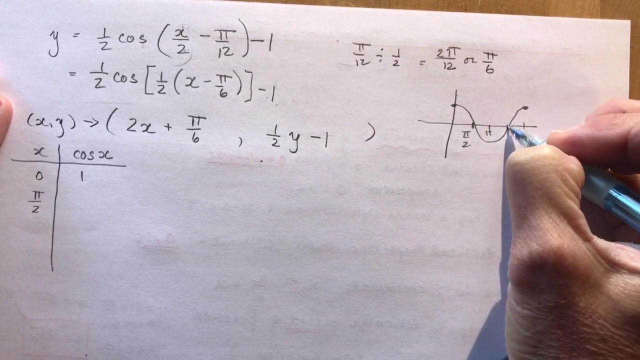 Let's draw it quickly right over here, So you go like: this Starts and ends here. Now remember, this is pi over 2 here, Sorry, 2 pi, This is pi, This is Pi over 2.. And this is 3 pi over 2.. 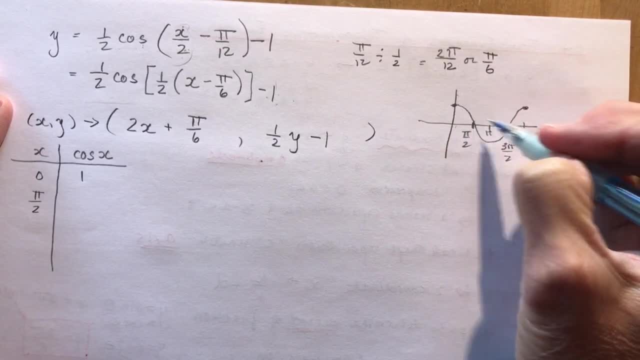 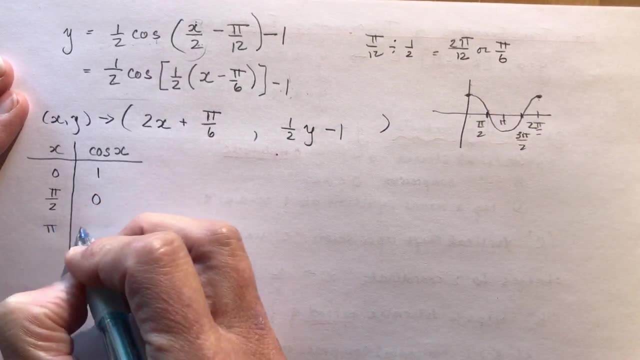 Okay, make a quick sketch And now you have 1,, 2,, 3,, 4,, 5 points that you can use. So pi over 2 and 0.. I have pi and negative 1. I have 3 pi over 2 and 0. 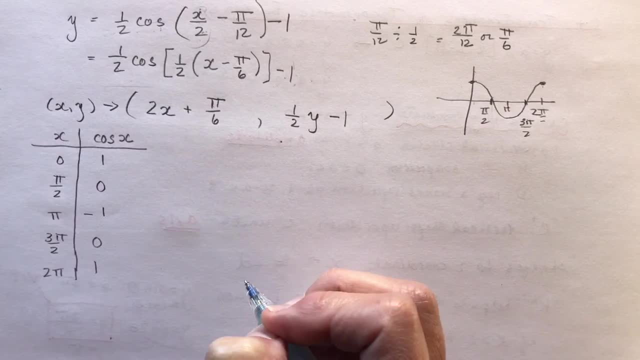 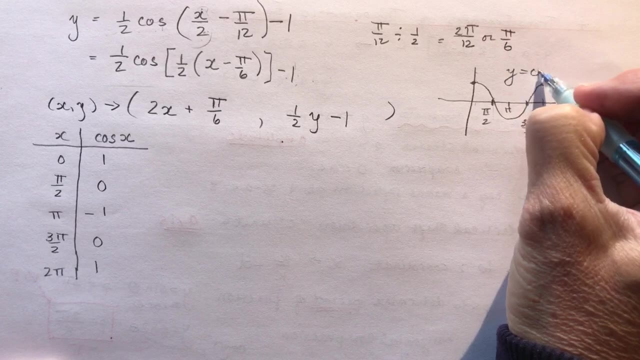 And I have 2 pi and 1.. Okay, so those were the. These are key points of the parent function. Right Y, equal Cos, theta, That's all Okay. so I want to do these transformations to these points. 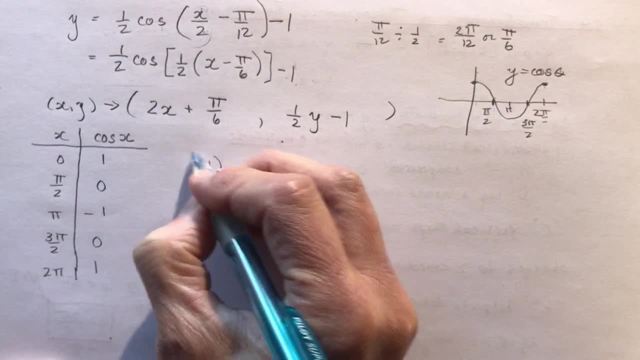 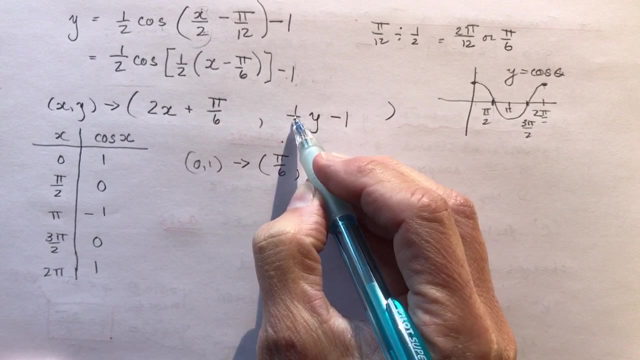 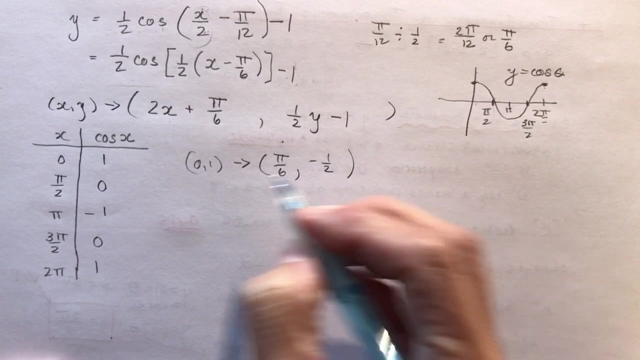 So I'm going to do 0,. 1 goes to And I'm going to plug in: x is 0 here, So that gives me pi over 6.. And a half minus 1 minus 1 half, Okay. and then we're going to do pi over 2 and 0. 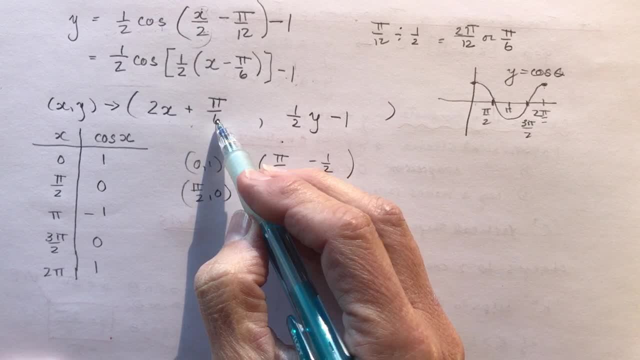 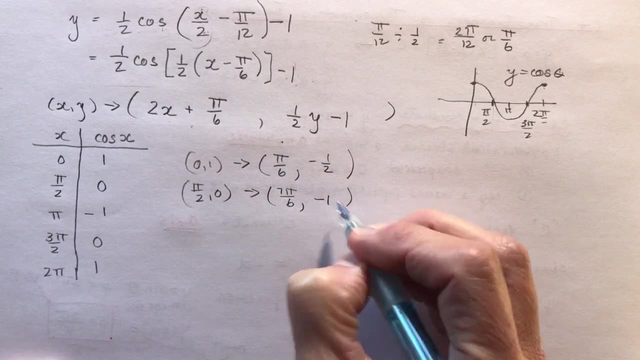 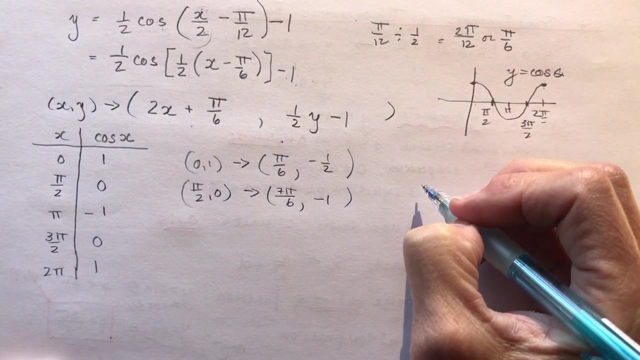 So pi over 2 times 2 is pi plus pi over 6.. That's going to be 7 pi over 6 and minus 1.. Okay, so what is our, What's our period? Let's do that, because that's really a good thing to know here. 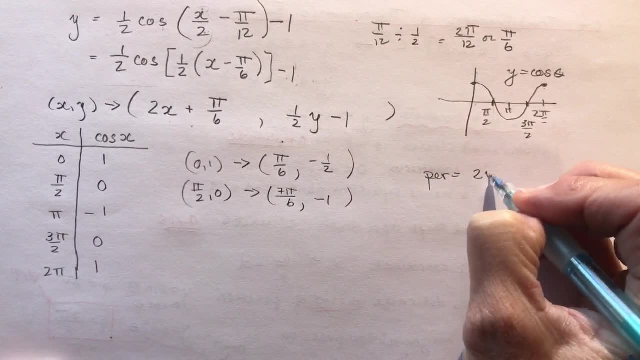 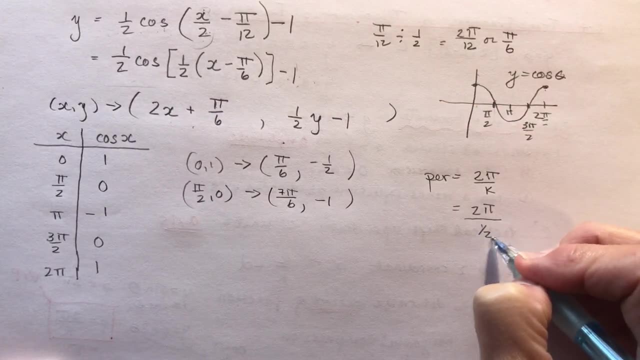 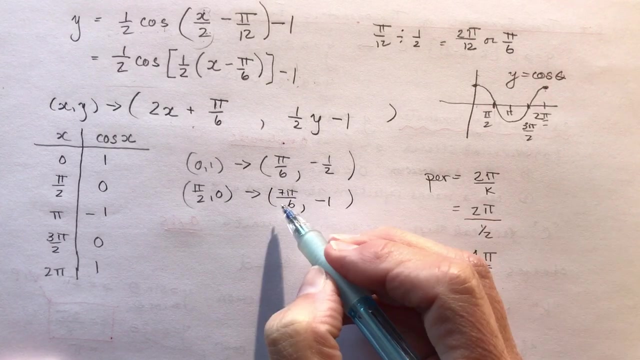 So period is equal to 2 pi over k, So that's 2 pi over. My k is a half, So that's 4 pi, 4 pi for my period. So I'm stretching it. That's why all these points look like they're so far apart. 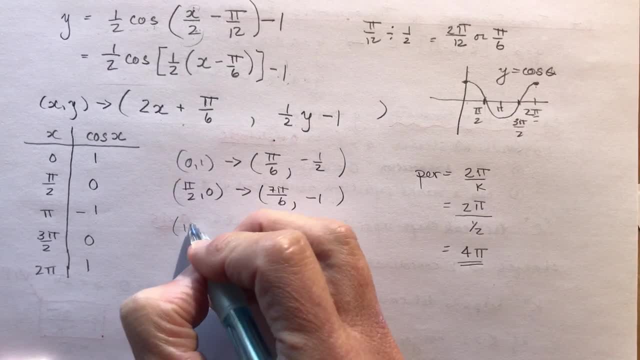 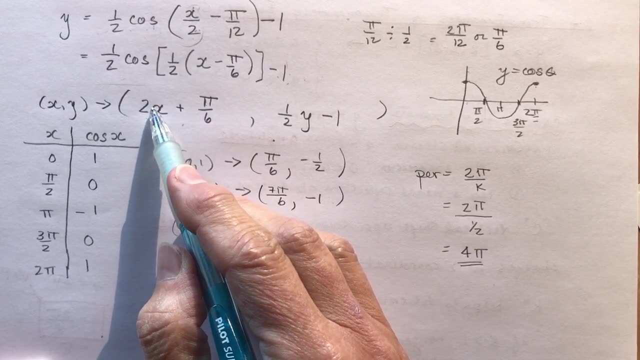 Right, Okay, so pi over 2. Let's go to pi and minus 1. So pi, that's 2 pi plus pi over 6.. 2 pi is 12 pi over 6. And one more pi gives me 13 pi over 6.. 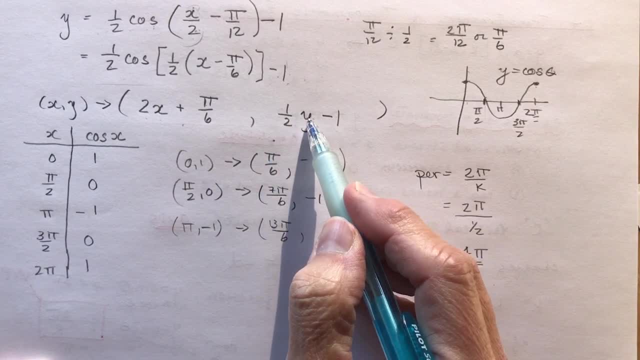 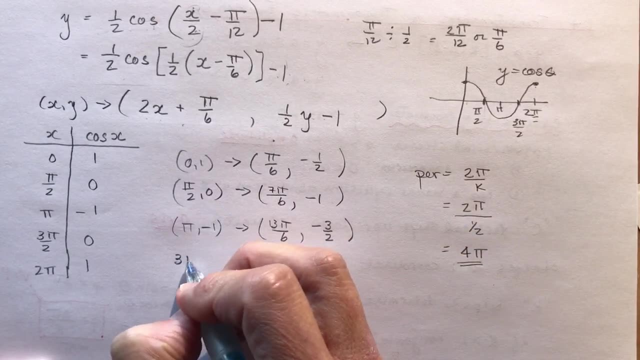 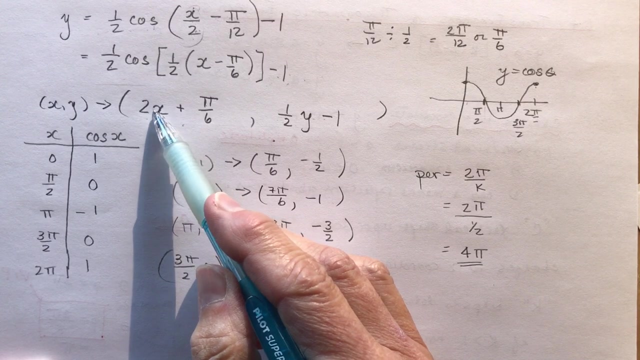 And minus 1 here for my y. So minus a half Minus 1 is minus 3 halves And then I have 3 pi over 2 and 0. And that gives me 3 pi over 2 times 2 is 3 pi. 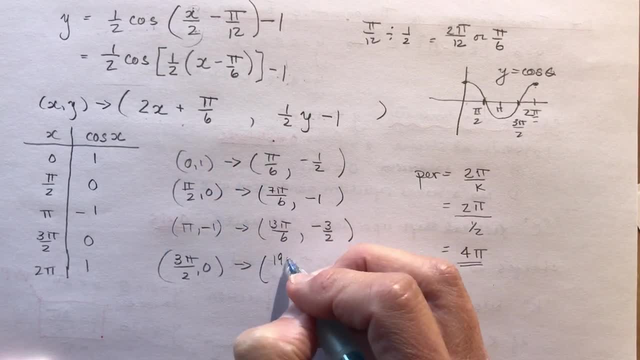 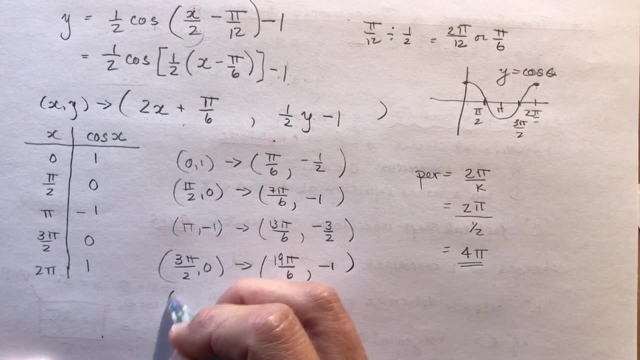 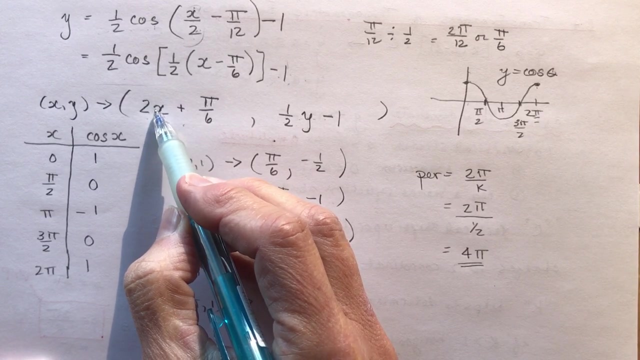 That's 18 plus 1 is 19 pi over 6 and 0.. Gives me minus 1.. And finally I have 2 pi and 1.. I transform that 2 pi, here goes 4 pi 4, that's 24 over 6 plus 1 more is 25 over 6.. 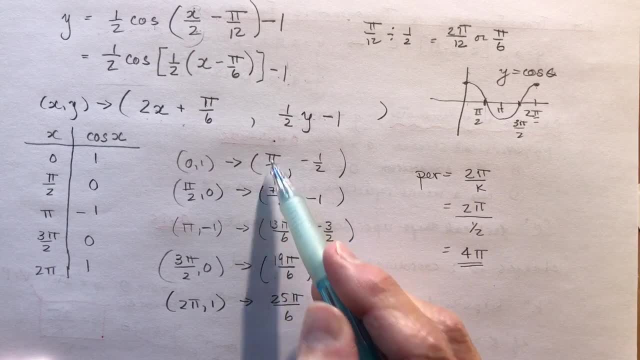 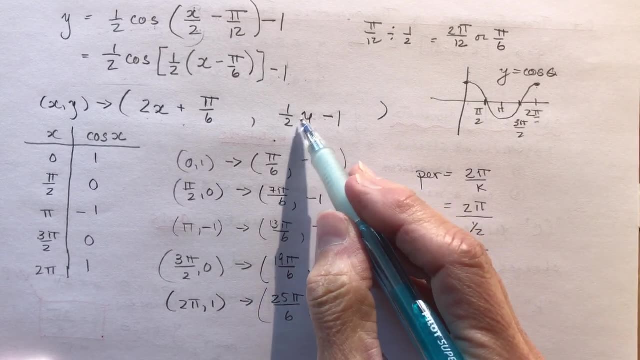 25 pi over 6.. You can see they're going up by 6s here right: Pi 7,, 13,, 19,, 25.. Probably have done that in your head a little faster, And a half minus 1 is minus a half. 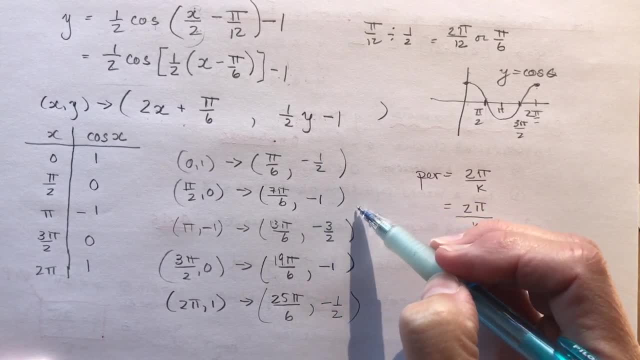 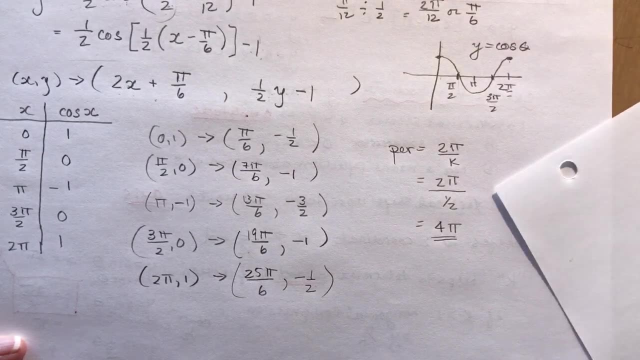 So you can see I've gone from minus half minus 1, minus 3 halves minus 1, minus a half, So it all looks really very pretty, Okay. so what I want to do now is I want to graph this. 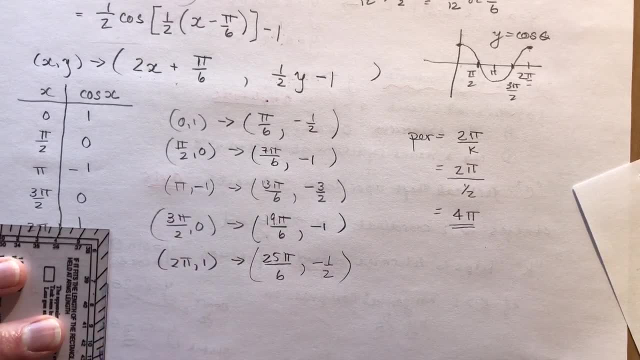 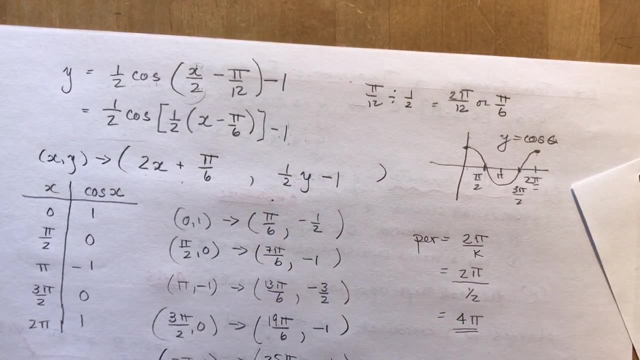 So I get out my trusty ruler here quickly. I usually like to have these graphs already done. Now let's take a look, first of all, where the axis is. Remember, this is your axis, right here Axis. So I'm going to be below. 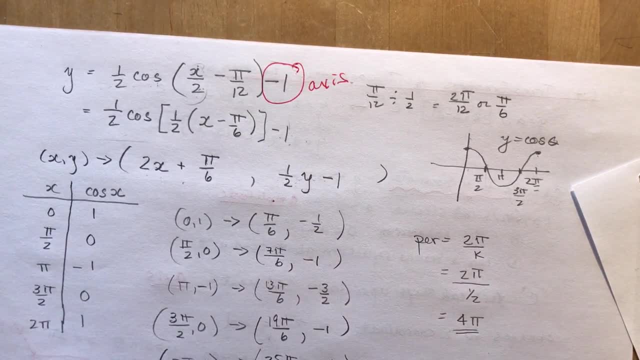 So I'm going to make sure when I draw my graph. I don't have, I'm not going to go off the page here- So I want the axis to be at Minus 1.. So let's call this minus 1, right here. 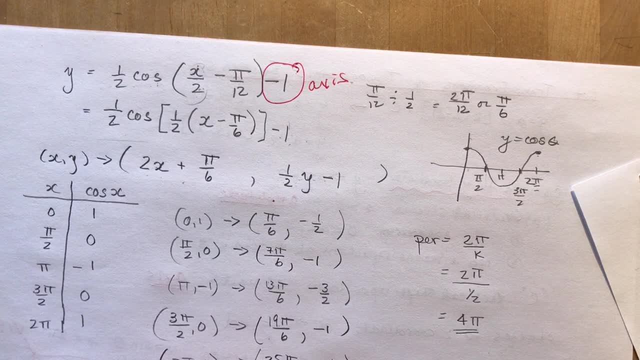 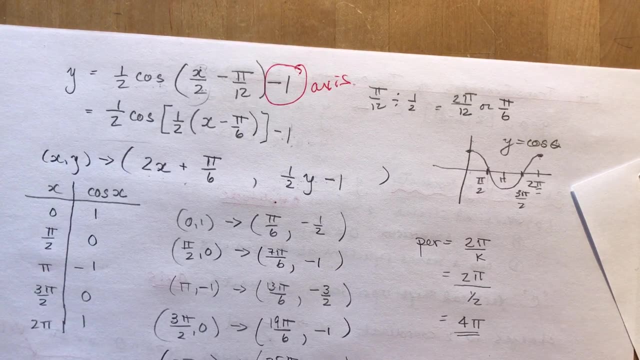 And I didn't give you a domain, But let's say it's between 0 and 2 pi, Which is what we've done. Okay, so this is: y equals minus 1.. We've got our axis down here, Oops, sorry. 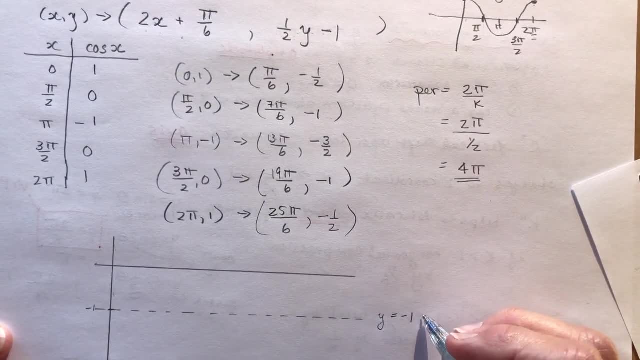 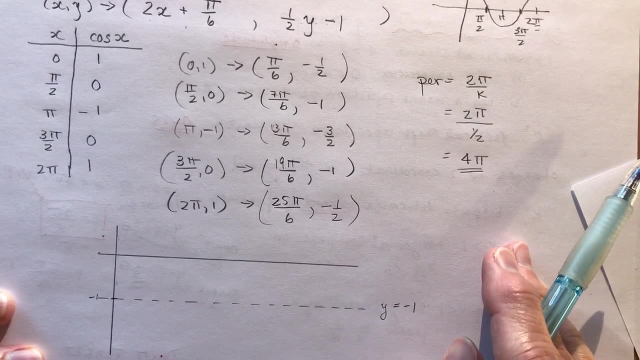 I guess I couldn't see that. And now I'm going to check out my amplitude. So the amplitude is 1 half. We have 1 half cos. So I'm going to- I'm going to be going up a half from here. 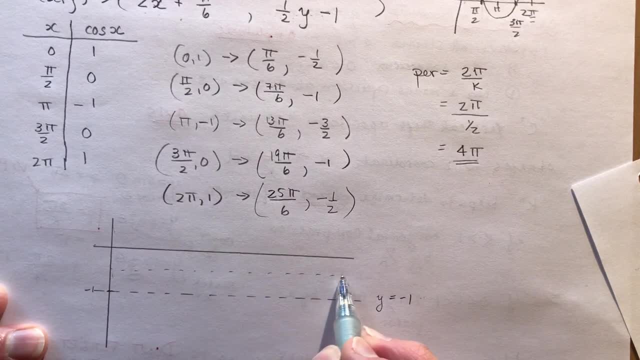 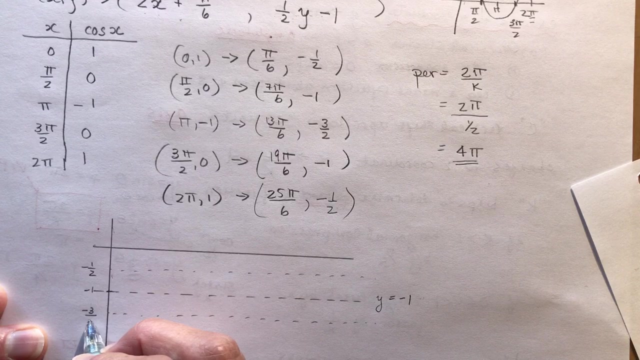 So this is the highest point on my graph And the lowest point is going to be another half below. This is always a good idea to do this. I mean it just gives you a little better sketch- Minus 3 halves, And you can see all my points go between minus 1 half and minus 3 halves. 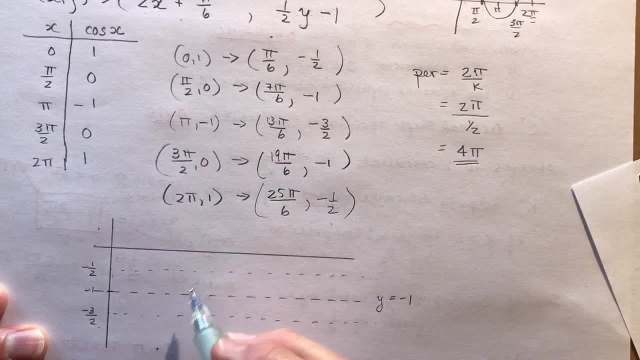 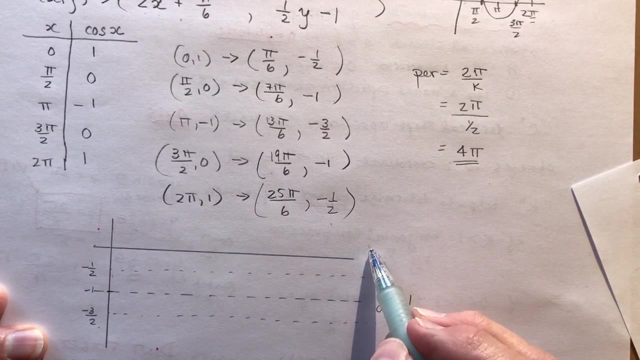 So now I've got- Um, I have to go back up here to give me my x-axis scale, So I'm going to shift it to the right: pi over 6.. So this is pi over 6.. We shifted it to the right: pi over 6.. 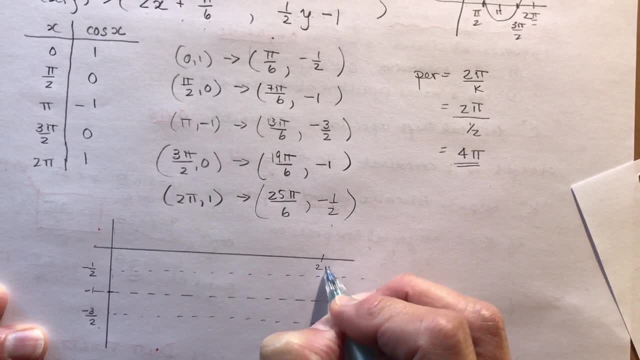 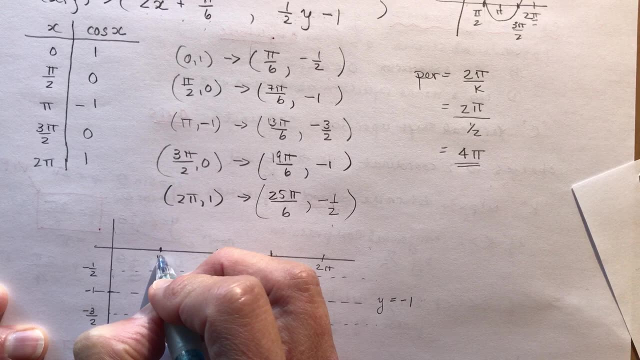 So let's say I make this 2 pi here. I'm going to divide it nicely into quarters, Like I mentioned earlier. So this is pi over 2. And my whole graph is going to be shifted pi over 6.. To the right: 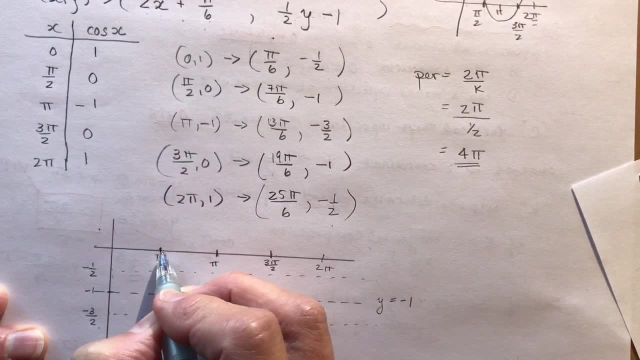 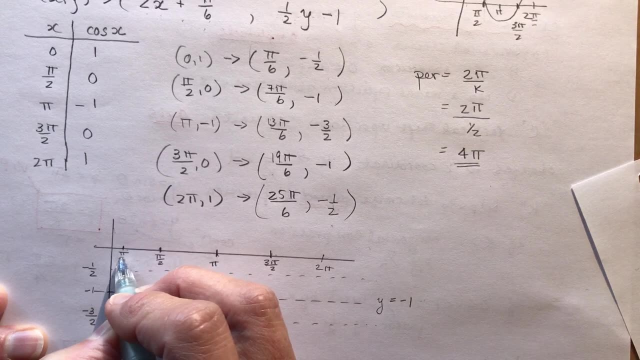 So that means I'm going to start pi over 6.. This is pi over 2.. So I want another. So let's say this is pi over 6, right here, Pi over 6.. 1, 6,, 2, 6,, 3,, 6.. 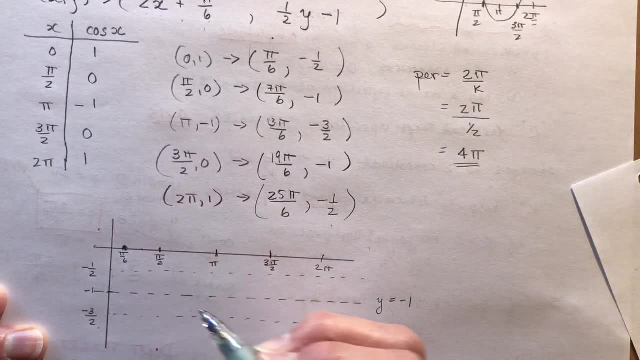 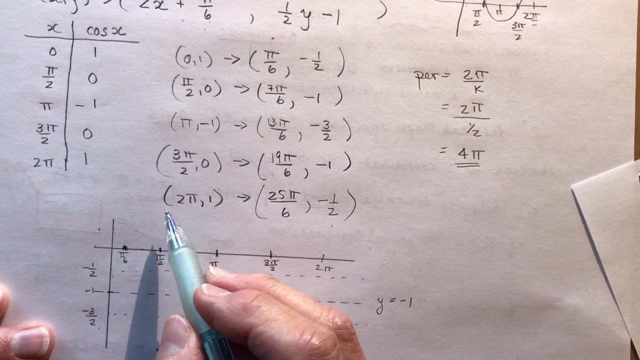 Yeah, it's about, Maybe about here. Okay, so pi over 6.. I'm going to start my graph there Now. the other thing you should note is that we have Um. Is this a positive cos function? Yeah, it was positive cos. 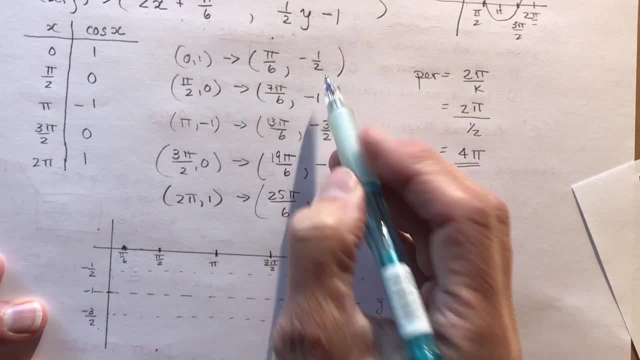 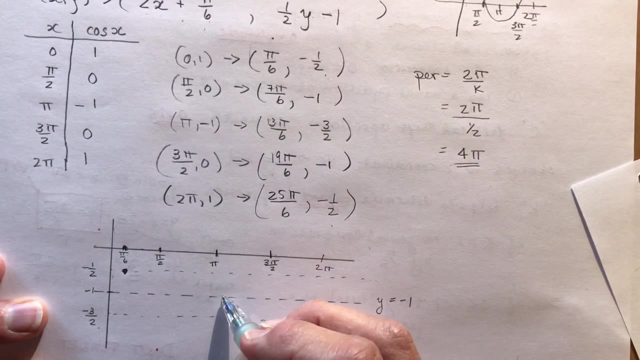 So we're going to start at the highest point, Which is what we are at here. So we're here, And then 7, pi over 6. That's just pi over 6. Away from pi, And we're at minus 1.. 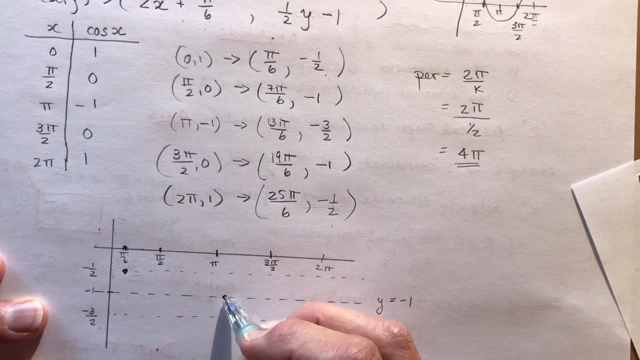 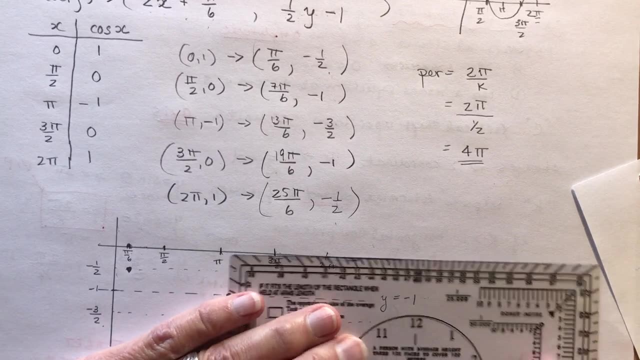 So that's here, And then 13 pi over 6.. So we have to stretch this right, Because we're going up 4 pi. Oops, Should have drawn my graph a little bit longer. Okay, So we have pi over 6.. 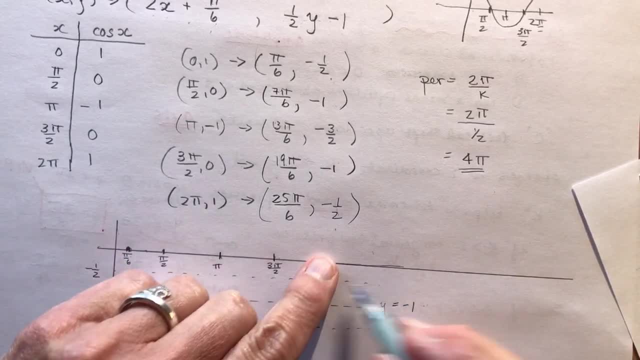 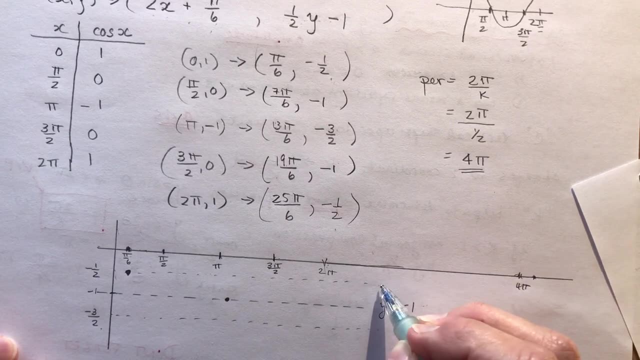 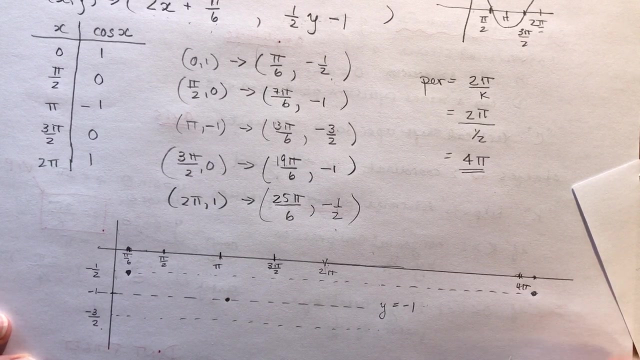 7 pi over 6.. 2 pi is that far, 4 pi is going to be this far Quick sketch And we're going to end here At 25 pi over 6.. My lowest point: This is minus 3 halves. 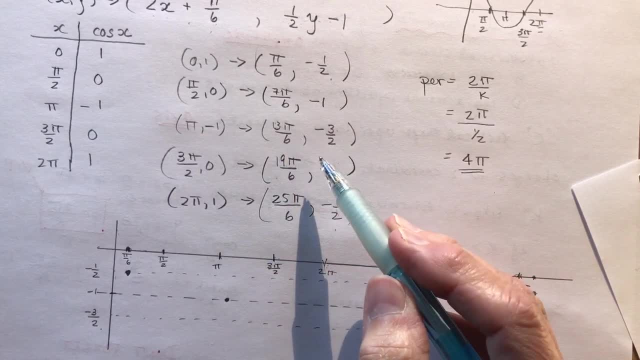 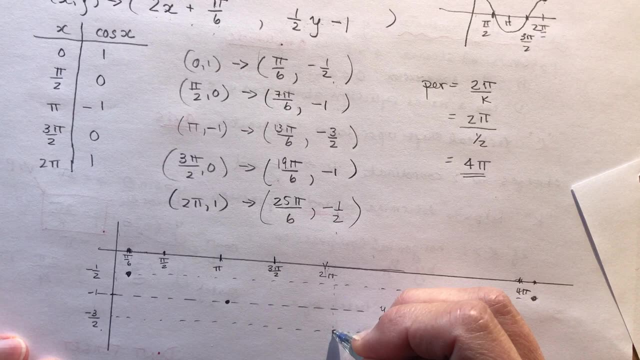 Is going to be at 13 pi over 6.. 13 pi over 6.. That's 2 pi Plus a sixth. So it's going to be right here. My lowest point, And I guess I should have made this: y equals 1 way over here. 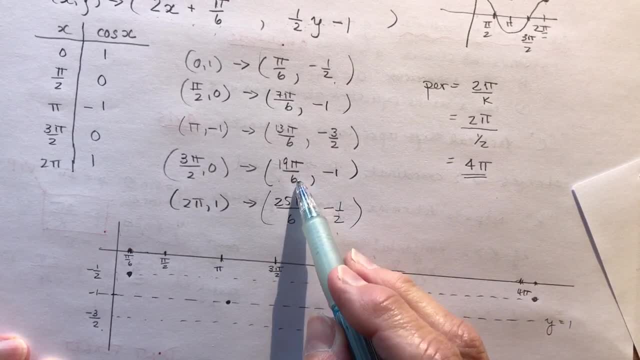 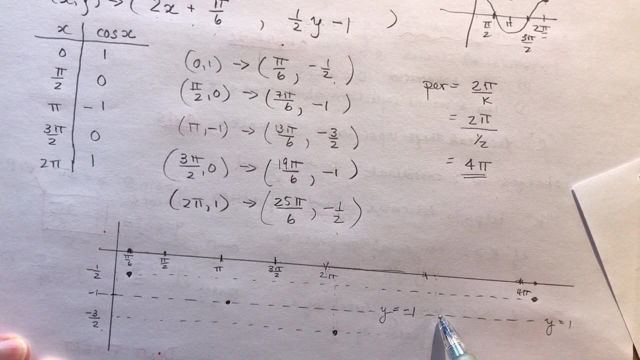 Instead, right in the middle of the graph, This one is going to be at 19 pi over 6.. So that's 3 pi Plus a little bit. So that's my other minus 1 point. So if you sketched all this together, 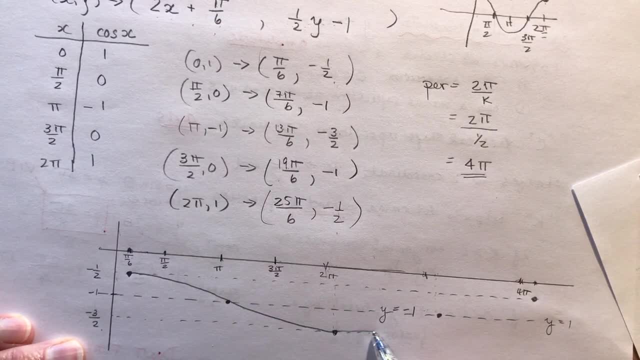 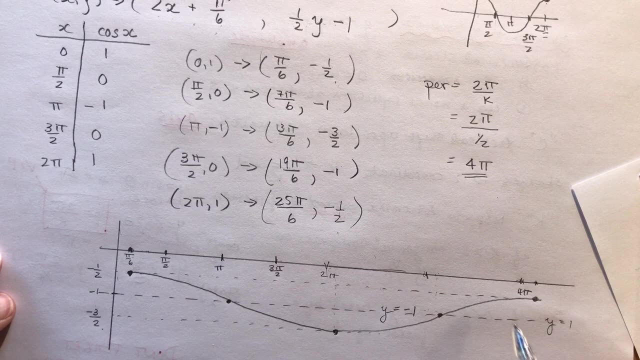 You'd have something going like this: Sometimes your graphs are almost flat. Don't be surprised If that happens. Okay, so there's my graph Now, like I said, You could make these points. This is always a good thing to do. 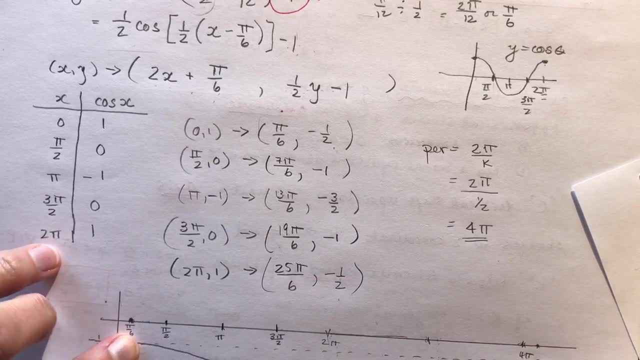 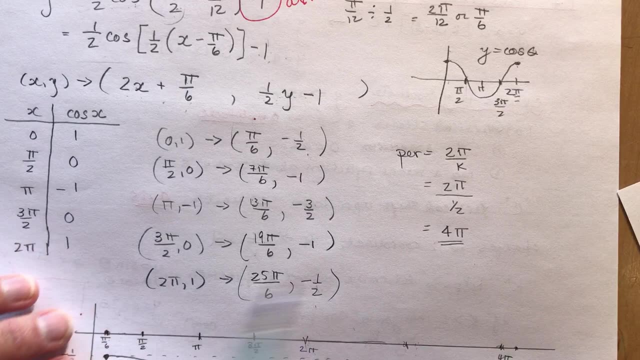 Know some key points: Do the transformations. Or you could have just stretched it out by 4 pi, Shifted it all over pi over 6. And done everything by quarters. I'm going to do that in the next example That I'm going to do for you. 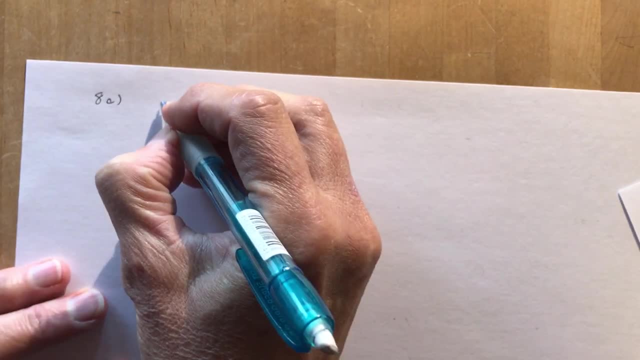 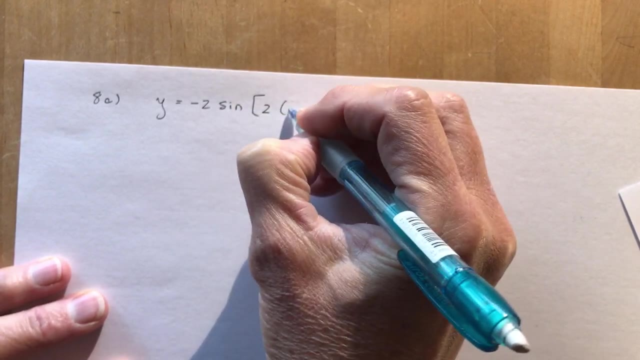 Okay. so the second one. This is from 8c, from your homework, In case your teacher gives it to you. It's done, Or at least an idea of how to do it. So this one They've already factored out. 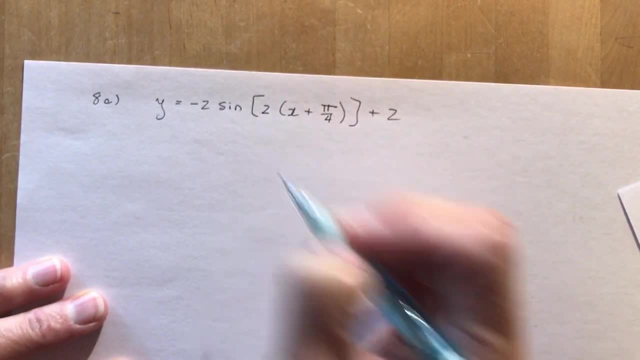 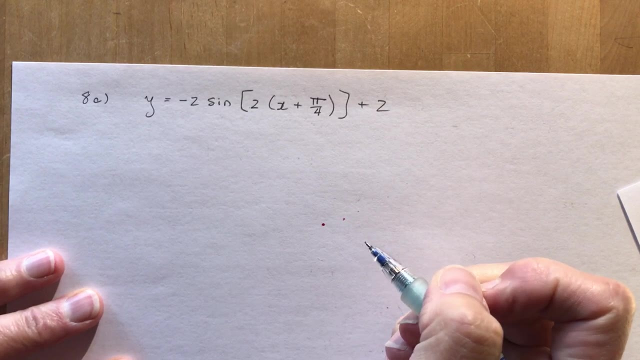 The 2.. So this is nice, It didn't have to factor it out And I'm going to, I'm going to sketch it just by, Just by sketching it. So let's figure out what the period is. first Period: 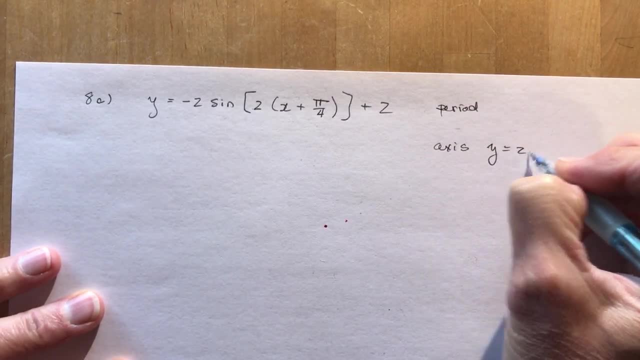 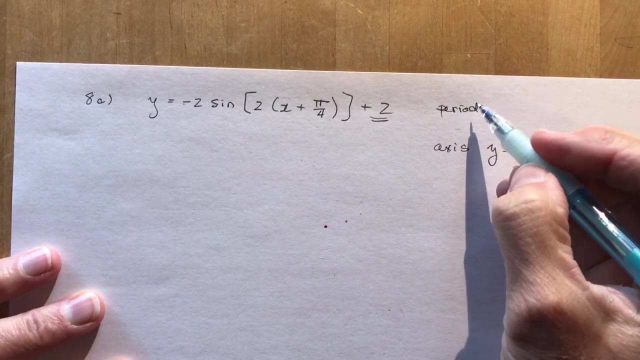 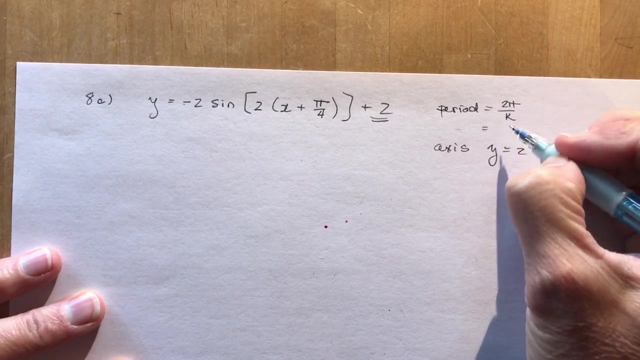 The axis. Axis is easy: Y equals 2.. Right in front, And this is: It's a negative sine function. And let's go back to the period. So it's 2 pi over k And in this case It's going to be 2 pi over 2.. 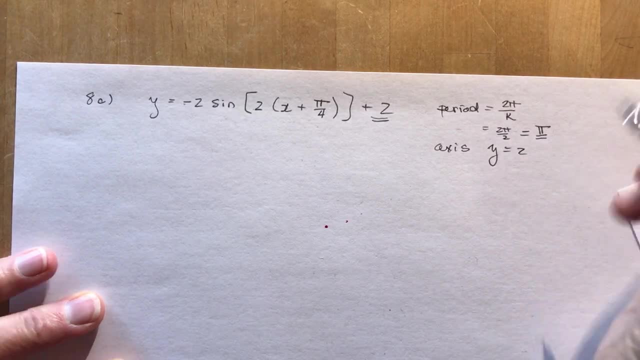 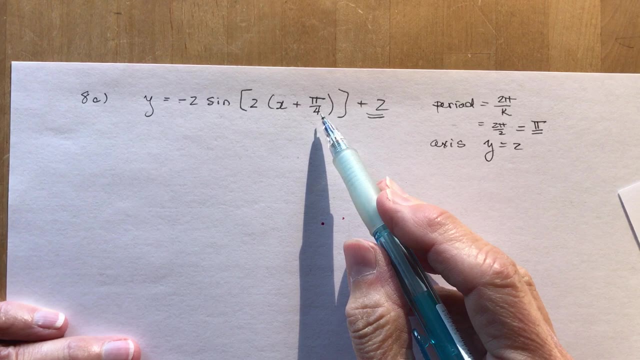 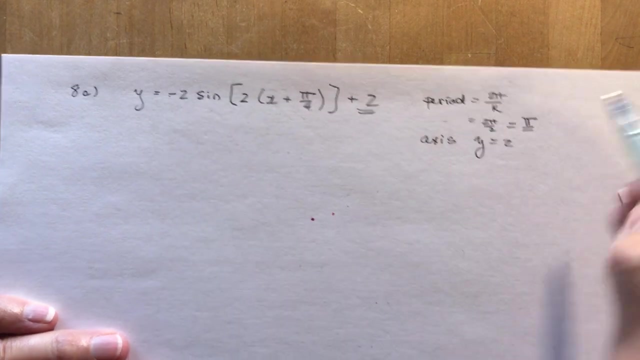 Which is pi. So We've compressed it Horizontal compression By a factor of a half Shifted to the left. Pi over 4. Axis is at y equals 2.. It's a negative sine function. So quick sketch. 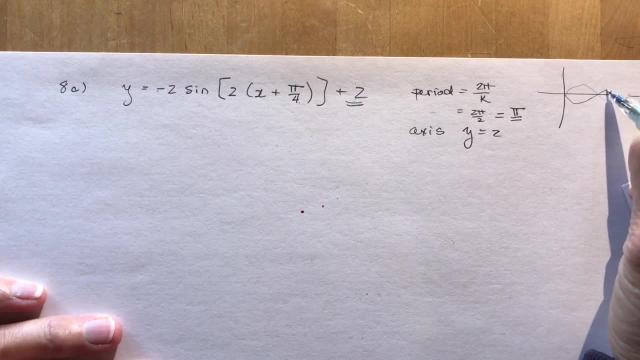 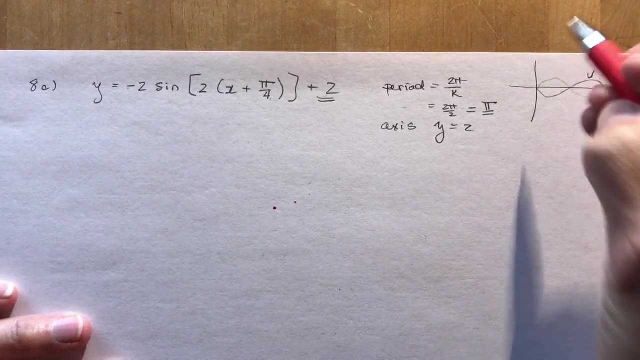 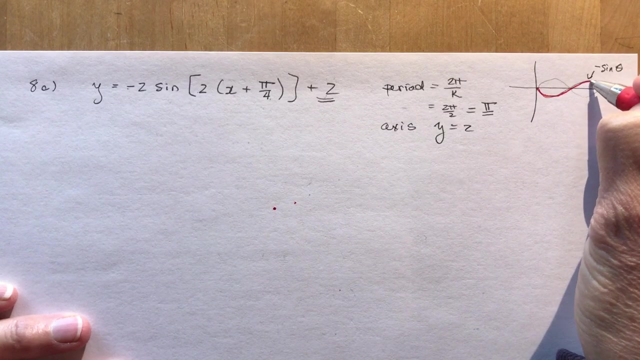 Here's your positive sine function. Right, So this is a negative sine function, So it's going the other way. Negative sine theta. Okay, So I'm going to write that in red here So you can see You really have 4 graphs to think about. 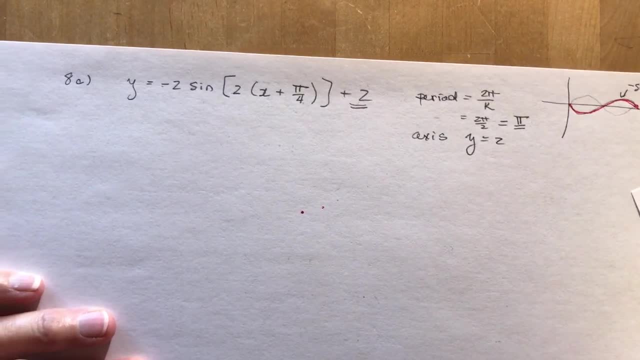 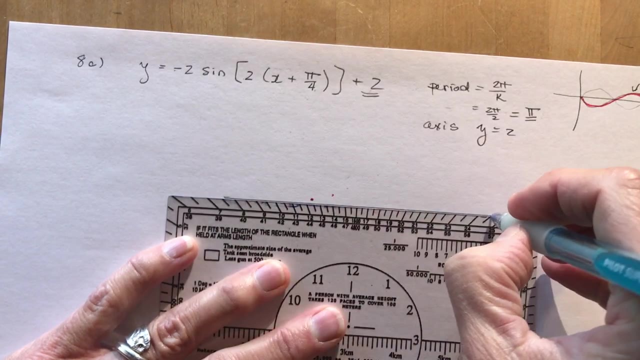 Positive and negative cos and sine functions. So it should look like that when I'm done. Right, So you don't have to draw it Without doing a mapping rule. You can do both If you want. I'm just going to sketch it like this. 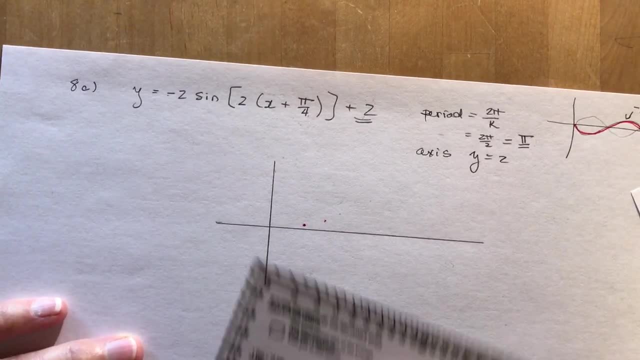 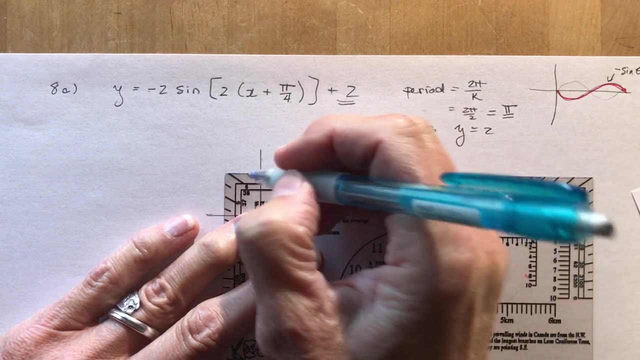 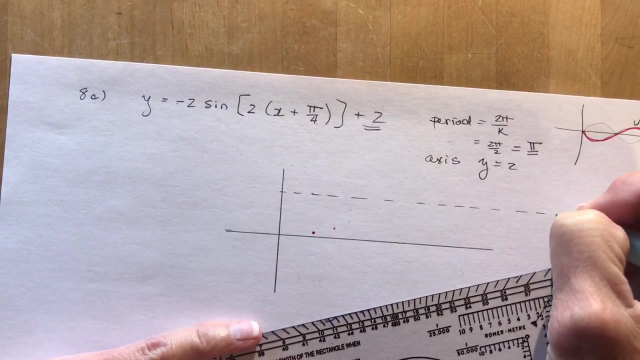 Okay, So My axis is at plus 2.. So first thing you want to do is Make a plus 2 here, So we write that on right away. Got our axis: Y equals 2.. Now my period is only pi. 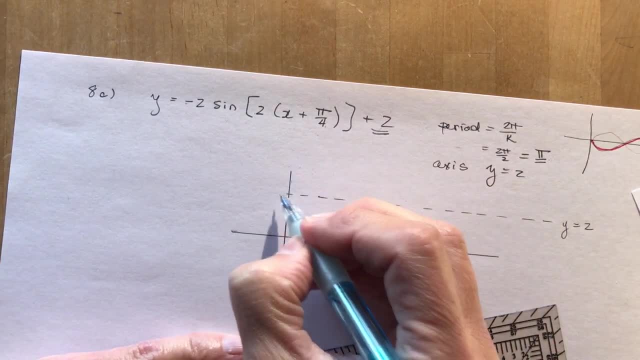 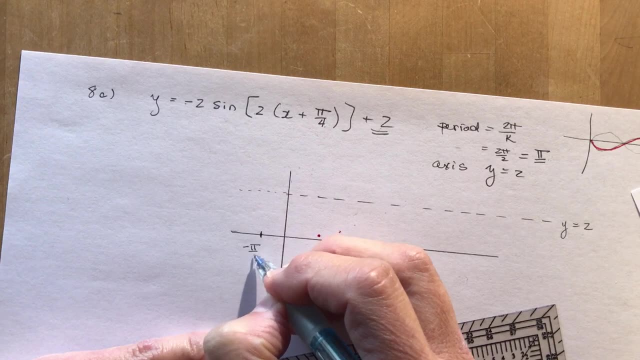 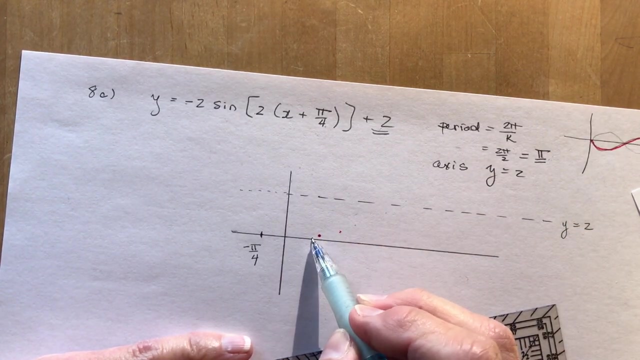 And I'm shifting it to the left: Pi over 4.. So where should I start To the left? pi over 4.. So I want to start at minus pi over 4.. The period is pi, So that means This is a quarter of a pi. 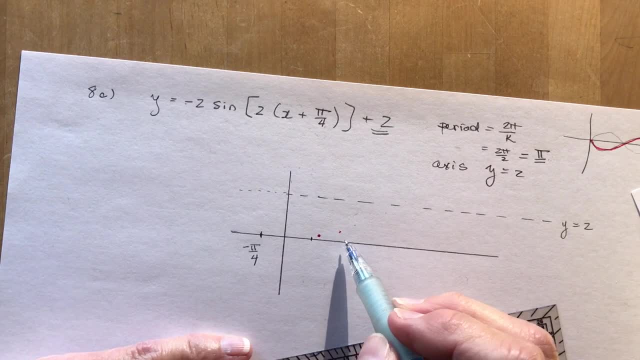 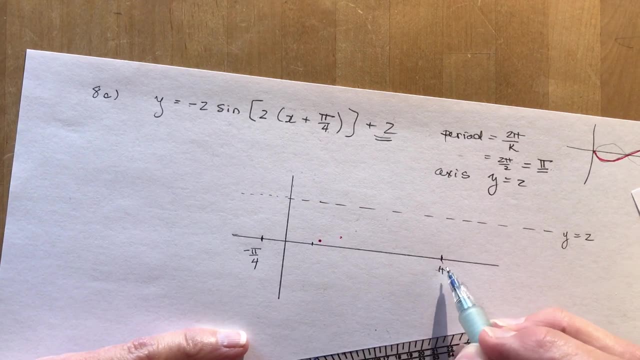 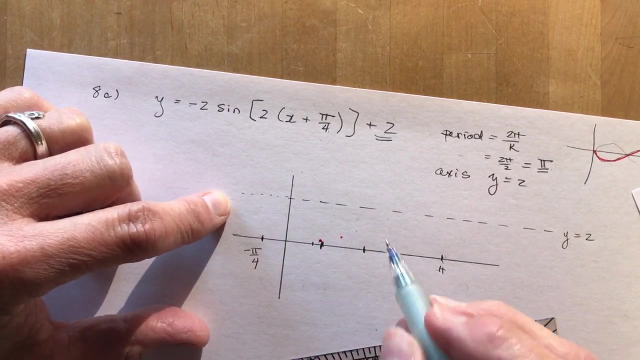 Is another quarter Here's. I should have made it a little farther apart, Maybe. So we're only going to pi All this pi, And from here to here. That's half a pi, That's a quarter of a pi. 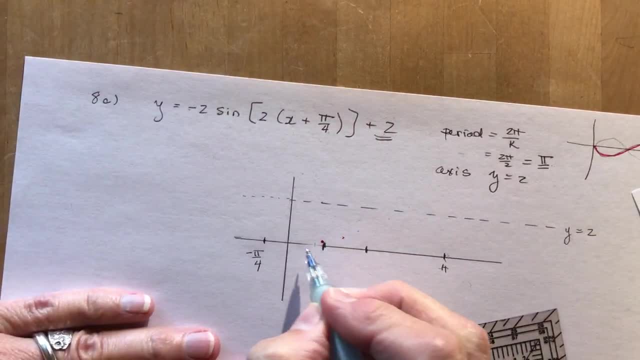 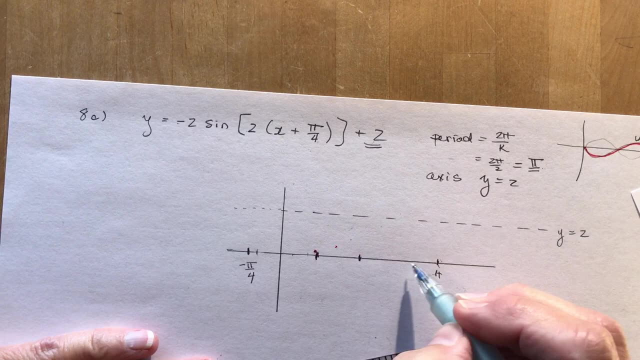 Let me just straighten this up a bit. I've got some red ink Came through on this. I'm going to move my quarter down just a bit So it looks more exact. This is a quarter pi, Half pi, Three quarters of a pi. 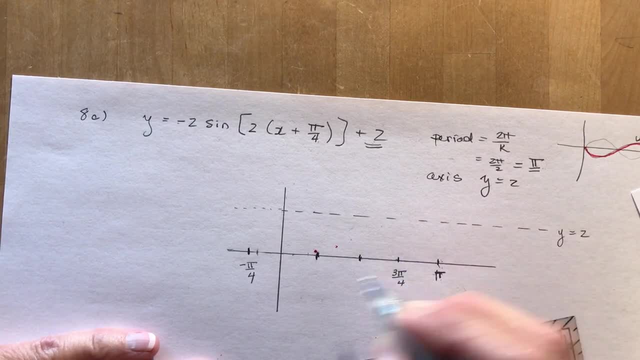 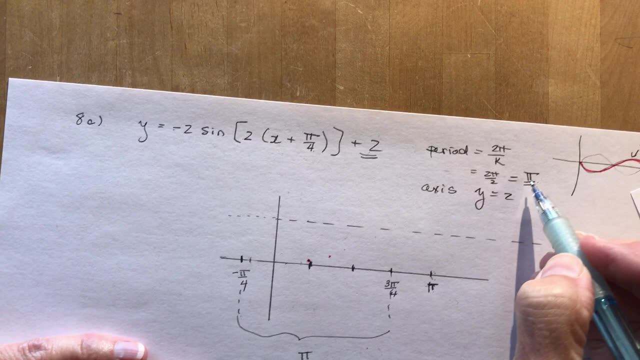 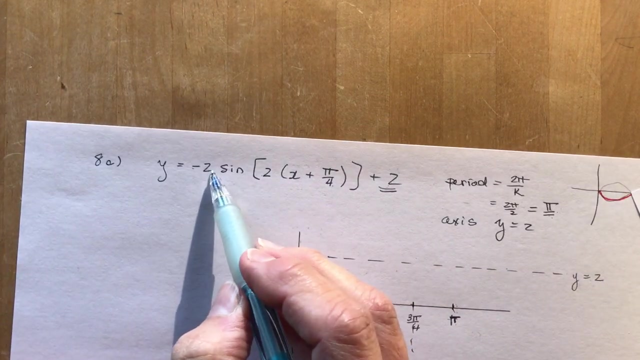 This is pi, But one complete cycle is going to end here, Right? So my period To here Is pi And my period is pi. Okay now, Because I have this, y equals 2.. And I'm looking at the axis here. 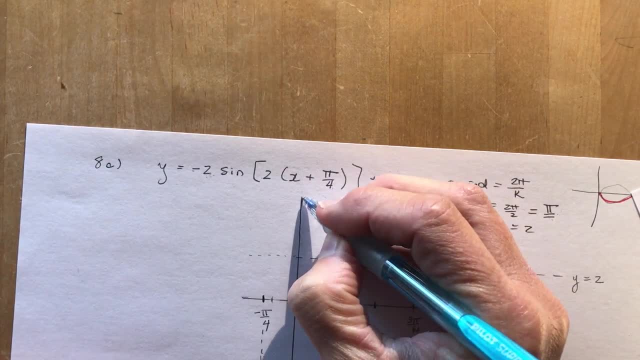 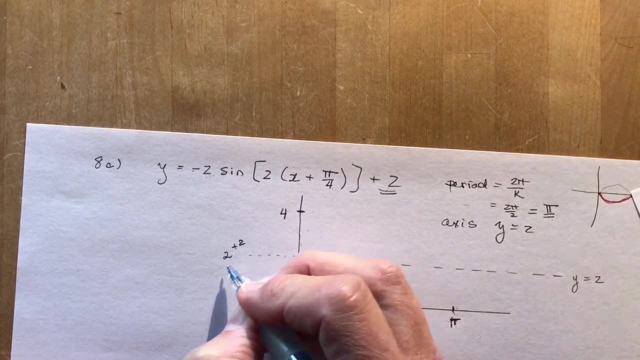 The amplitude is 2.. So I'm going to go up 2 from that. So this is a b4. And I'm going to go down 2.. So this is 2 plus 2.. 2 minus 2. Right. 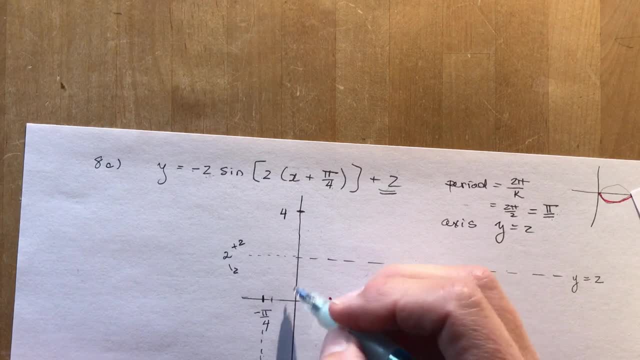 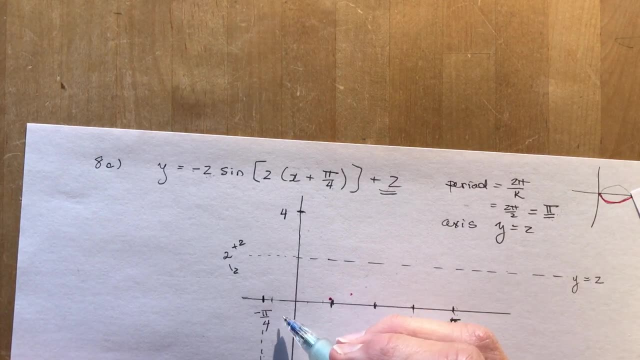 That gives me the total amplitude of my function. Not amplitude but the range. So the amplitude is 2.. So I'm starting at a negative sine function. So you always start a sine function on the axis, Don't start it down here. 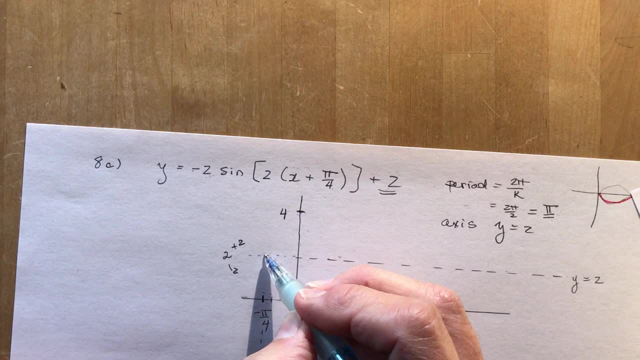 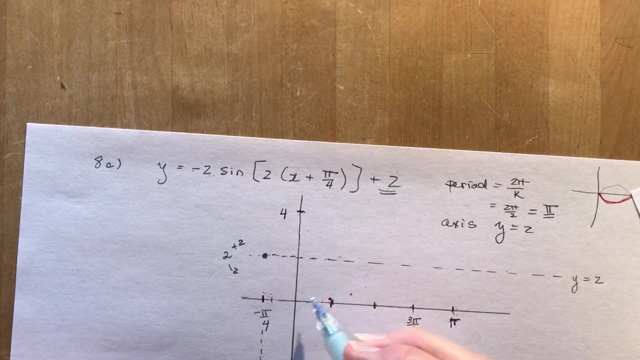 This is your axis here, So you want to start it right here? Okay, Start it on your axis. This is another thing. I get students that try to put it down here And then they don't know what to do, So I have. 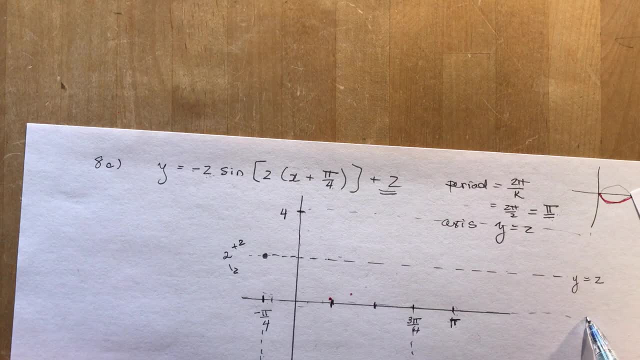 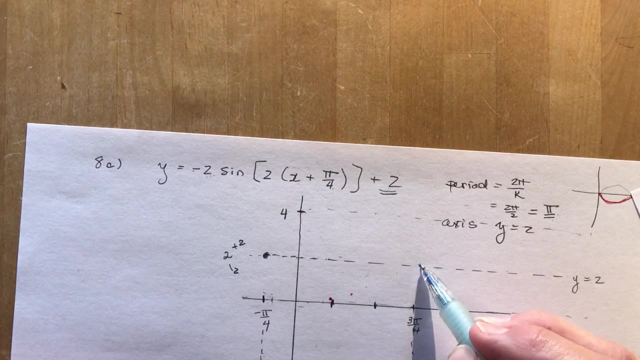 This is my maximum height. This is going to be my minimum height, Right? So it's a negative sine function. It's starting at minus pi over 4. And it's going to end here. That's one full cycle. If your teacher asks you for two complete cycles. 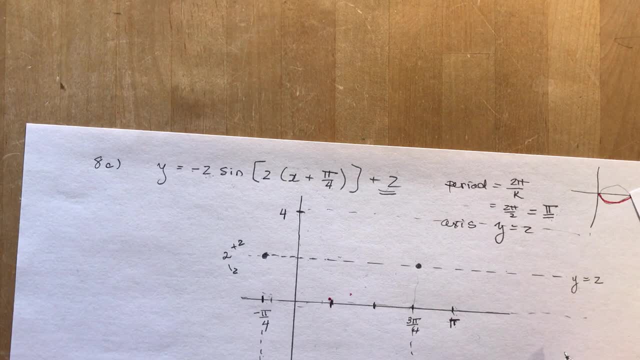 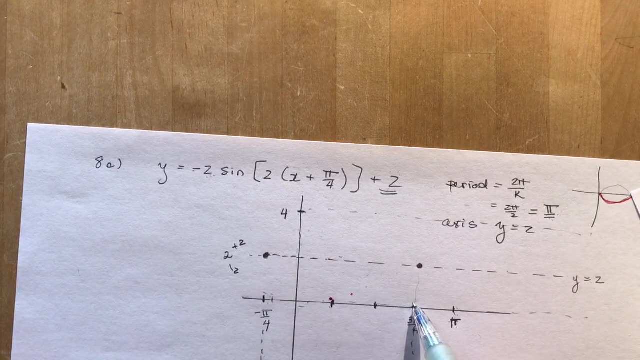 Well then you're just going to draw another cycle afterwards, Cut and paste it. Okay, So if I go from minus pi over 4 to 3 pi over 4.. Where is the lowest point? That's the lowest part on this graph. 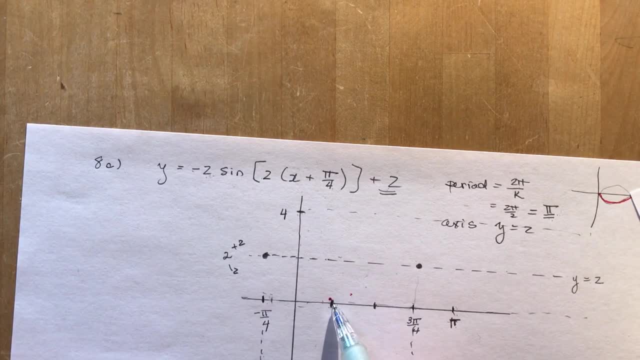 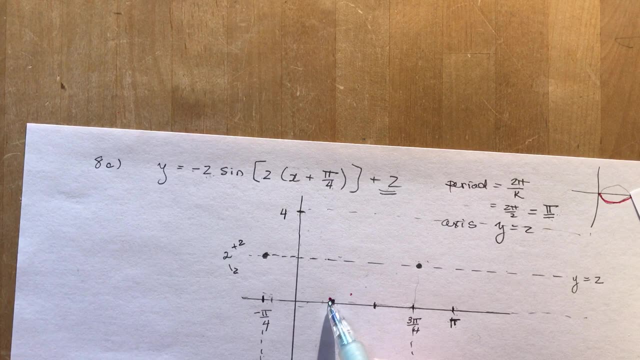 So 1, 2, 3, 4.. 1, 2.. Right here, This is going to be the lowest, That's the midpoint between the two maximums, And it's going to be right here on the graph. 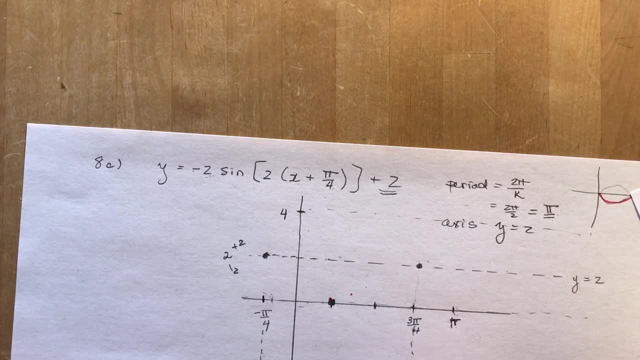 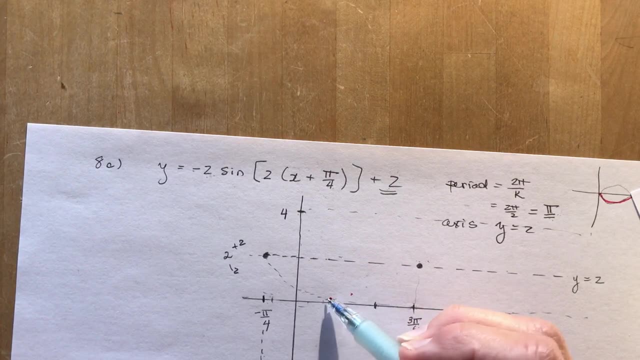 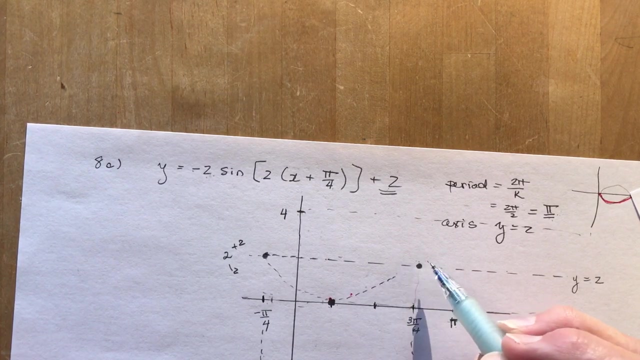 So I'm going from This way, Like this, Because it's going negative, sine It's going to go. Oops, I have to end at the. I have to end at 3 pi over 4. And I have to go up and down between them. 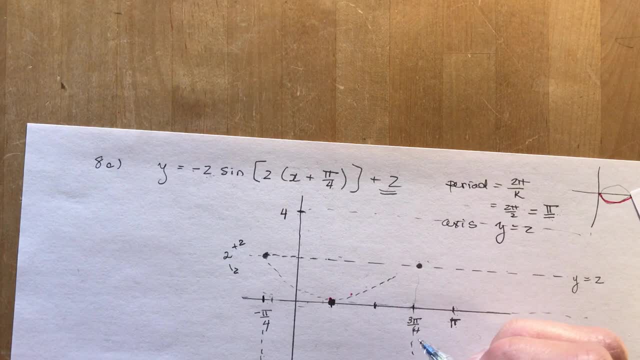 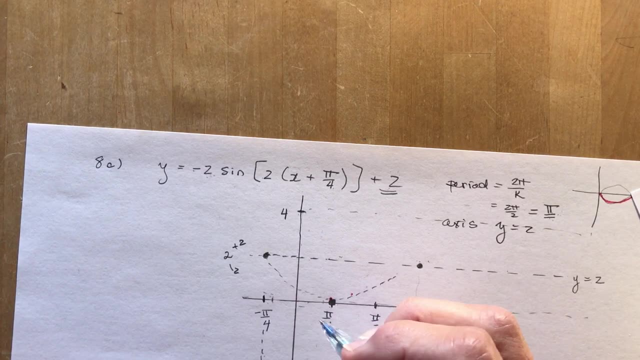 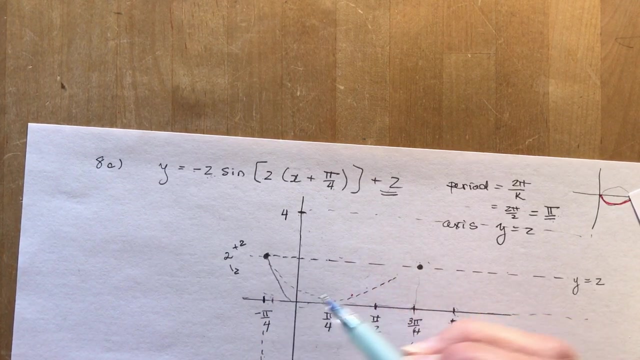 So pi over 4.. This is 3, pi over 4.. This is going to be pi over 2.. Pi over 4.. 0. So it's going to have to go through here. This is going to be my lowest. 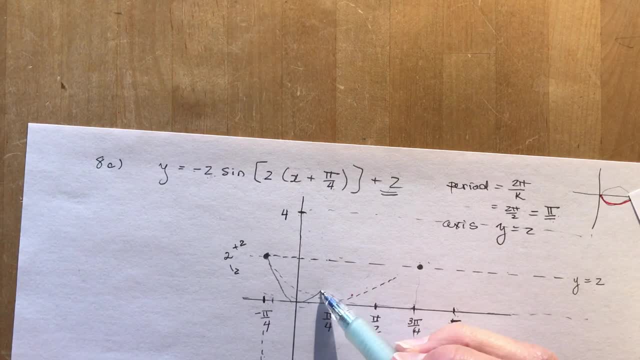 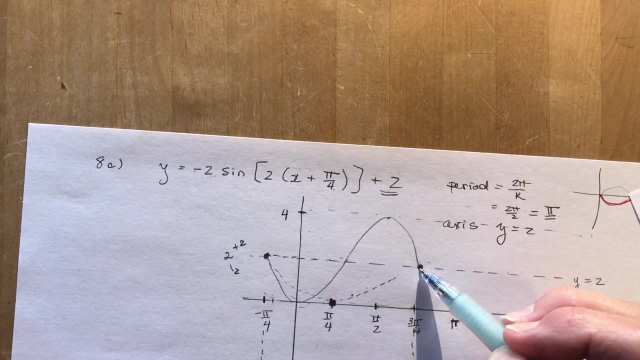 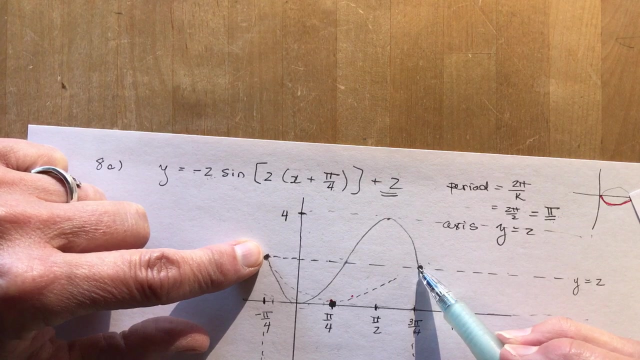 And then it's going to go Pi over 4. Here The highest point is going to be here, So you're dividing it into quarters And back down to here. So you have a starting and an end point, Right, This is pi units. 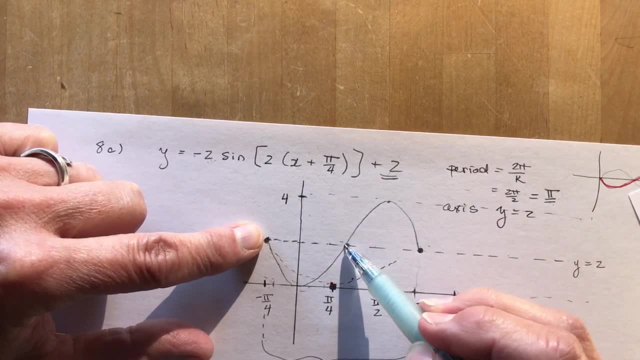 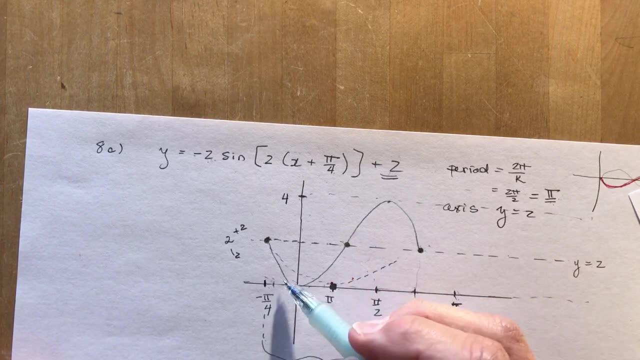 So go pi over 2 units And that's going to be back on the axis. So we have axis 3 points, The highest point at pi over 2.. The lowest point at 0.. And there's your sketch. Now you could keep going here. 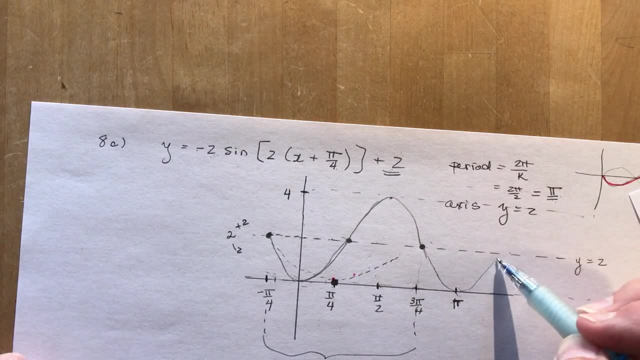 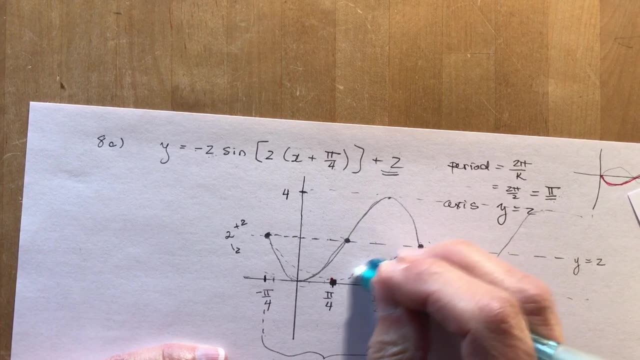 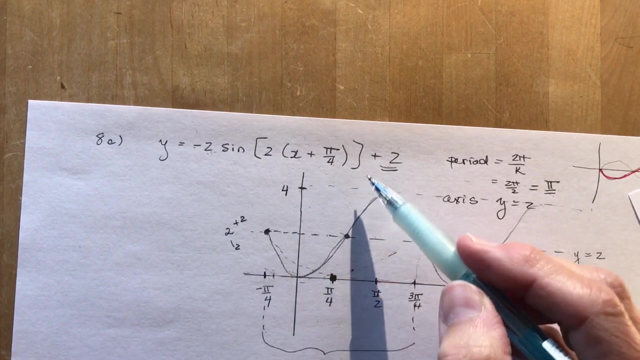 Right Like this. Depends on how far your teacher wants you to draw it. But you've got. What do I do this for? Okay, So there you go. There's your negative sign: 2x pi over 4 plus 2.. 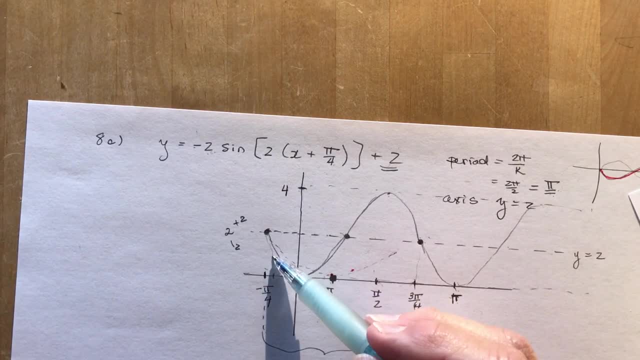 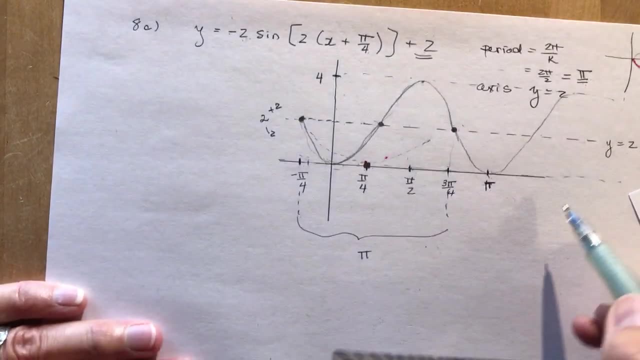 I've got my axis. I'm up 2, down 2.. I started on the x axis. It was negative sign. So I went down first And there's your negative sign function And say Let's just write out the mapping rule. 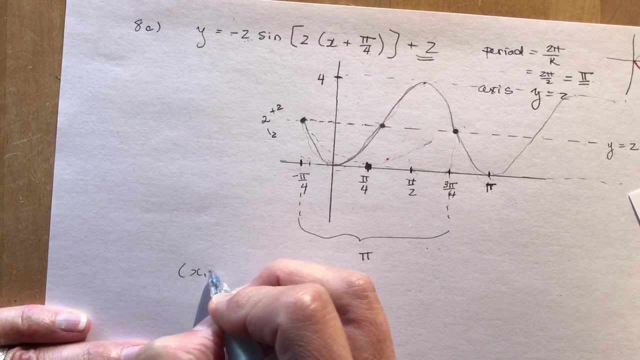 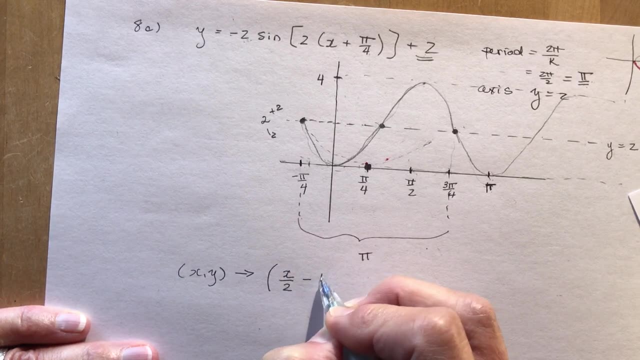 I won't do it all for you Because it's getting a little long here. But let's say we have x and y Go to. What do we do to the x's? So we have x over 2 minus pi over 4.. 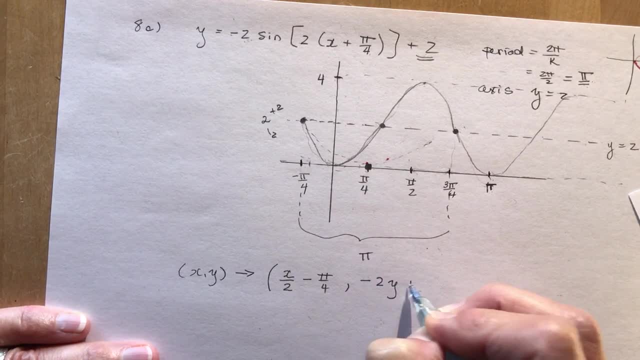 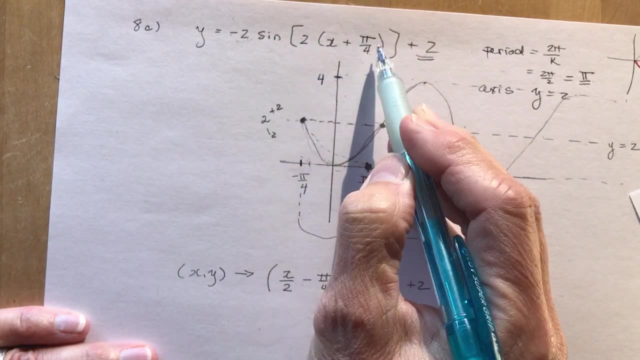 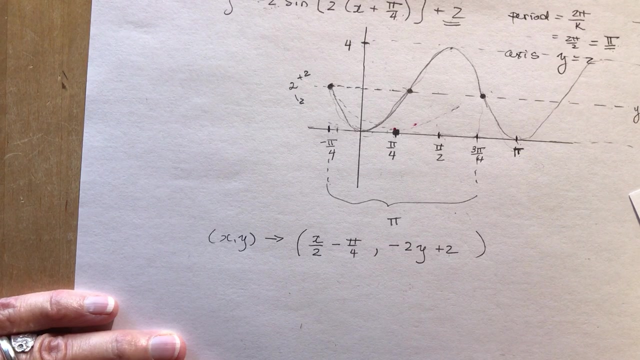 And minus 2y plus 2.. That's my y coordinate, See Minus 2y plus 2.. This divided by 2.. x divided by 2.. Subtract pi over 4.. And we use All the key points on the graph. 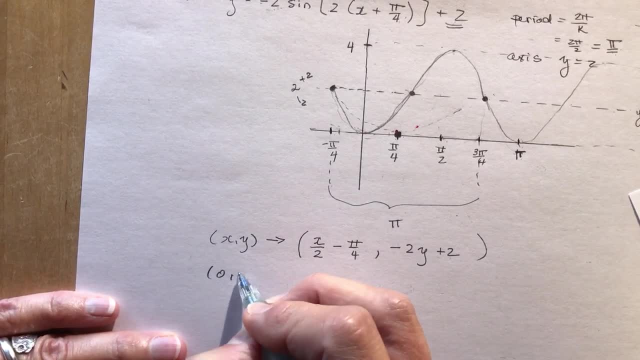 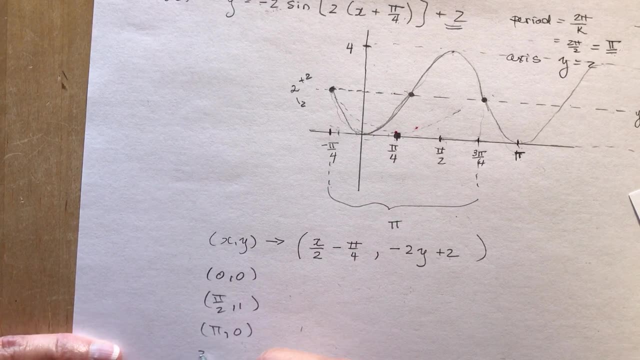 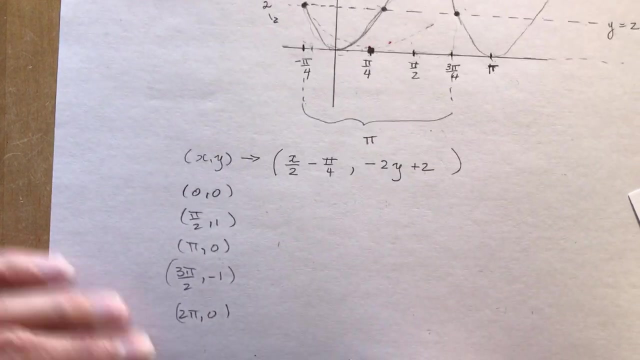 Of the regular sign theta. So I'll just write them out quickly here: 0,, 0.. Pi over 2. And 1. Pi and 0.. 3 pi over 2. And minus 1. And 2 pi and 0.. 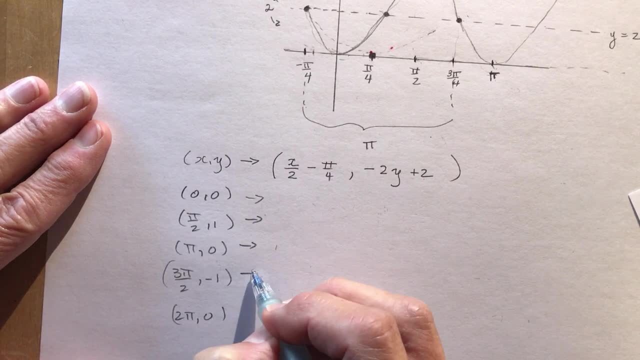 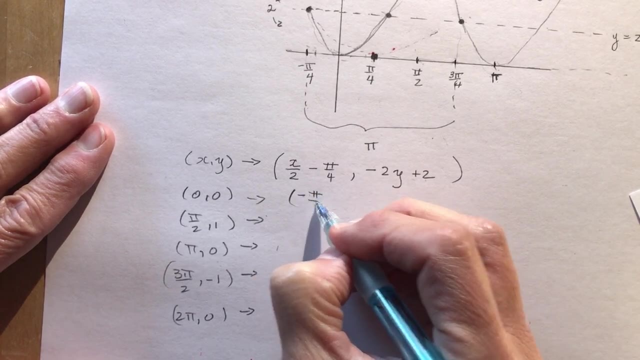 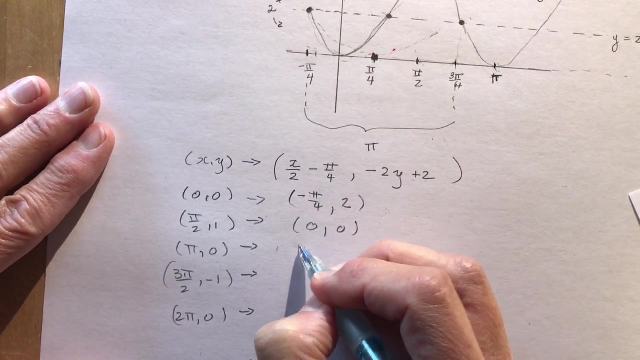 So you get all your points And then you apply all these, Get all the points Using these transformations. Okay, so We might as well just finish it here. Minus 4, pi over 4. And 2. This goes to 0 and 0..